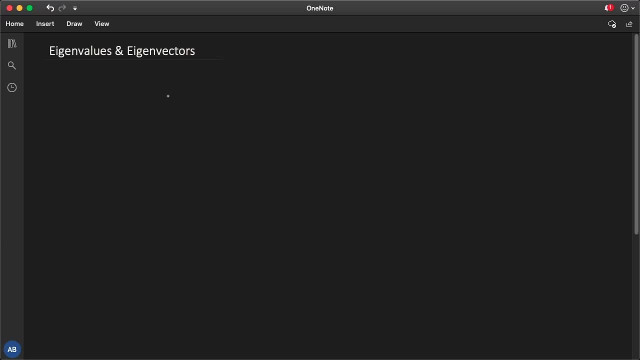 What is up you guys? So in this one we're going to be talking about a new topic called eigenvalues and eigenvectors. So this lecture and the next two or three are going to be around this topic. so just an overview of those lectures. Say, I've got a square matrix and eigenvalues are only. 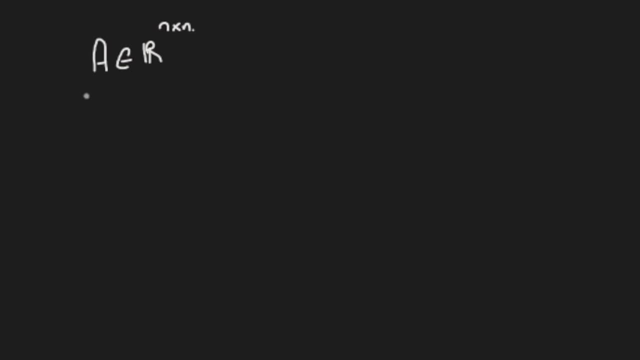 defined for square matrices. Now, for a large number of problems in engineering and science, it is necessary to find a vector v, such that if I multiply a by v, we get a scalar multiple of v. that said, we get lambda v, where v is a scalar and not a matrix. Okay, v is a vector and a is. 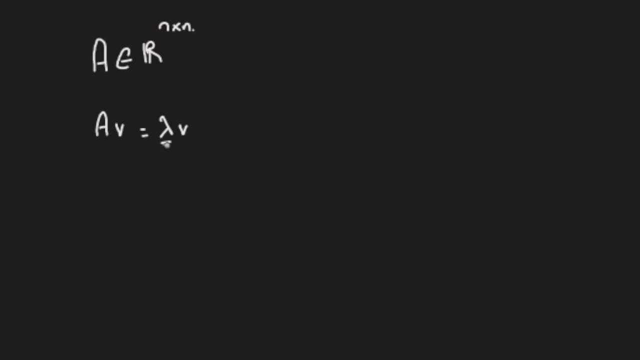 the matrix. So if you can find me a couple scalar, lambda and a vector, v. so lambda is a scalar and v is a vector, then guess what? You found one eigenvalue and its corresponding eigenvector. Eigenvalues and eigenvectors are always paired up, that is, for each eigenvalue there's a corresponding eigenvector, right? 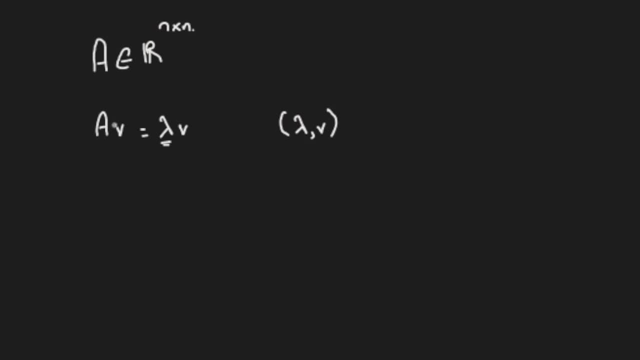 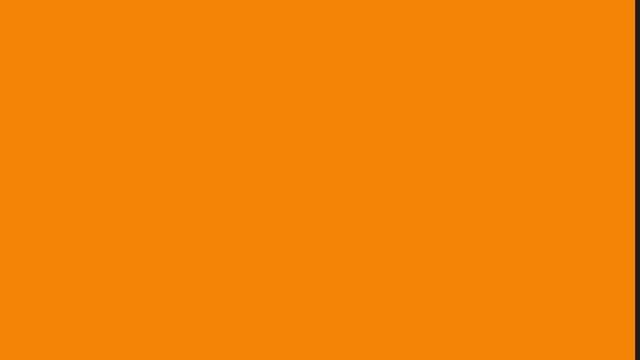 So in many problems in engineering and science we care about those quantities that characterize the matrix a. Now, graphically, what that means is that the vector a v- don't forget that a v is also a vector a v. so if, if, if, this is v and 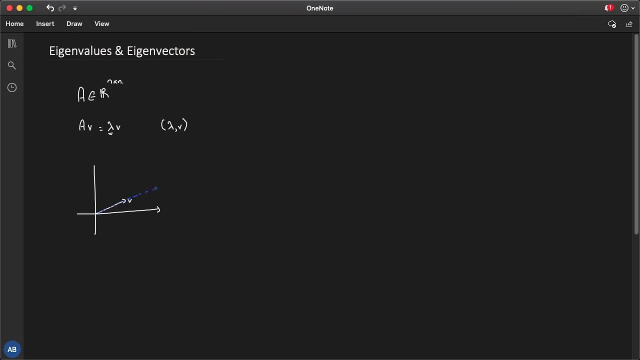 if we were to plot a v. in that case we say that a, v and v are parallel and lambda v only stretches and compresses v. So lambda v- if lambda is greater than one, it stretches v. let's say it's positive. so lambda v is going to be on this line as well. let's say it's somewhere here and compresses if. 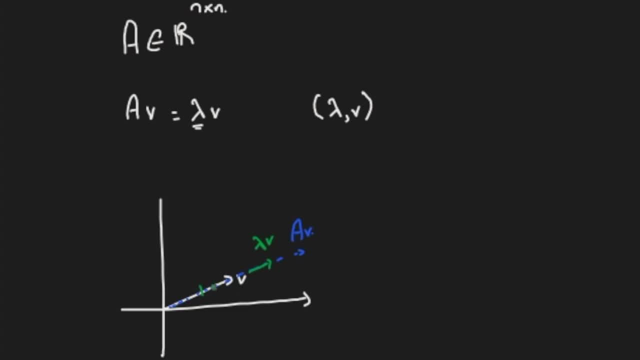 it's less than one, greater than zero. it lies here somewhere here, so lambda. v is compressing v and a v is still parallel to v. actually, in this particular example, it coincides with v, so graphically, this is what it means: v is a vector that first of all, preserves the direction of v. 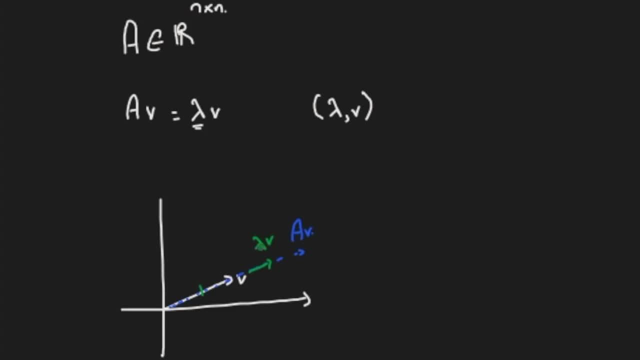 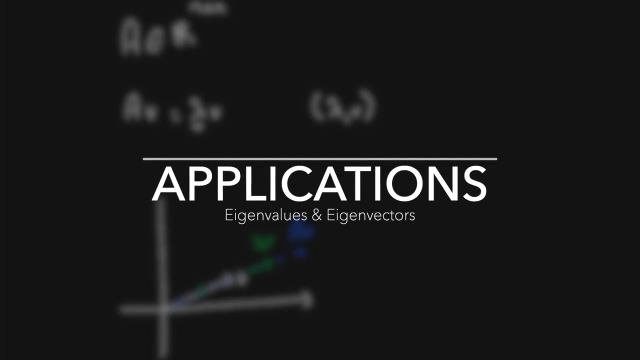 and second of all, it either compresses or elongates the vector v, in other words, it doesn't rotate v. so the value lambda here is an eigenvalue of the eigenvector v. it is worth keeping in mind that computing eigenvalues and eigenvectors is one of the most important. 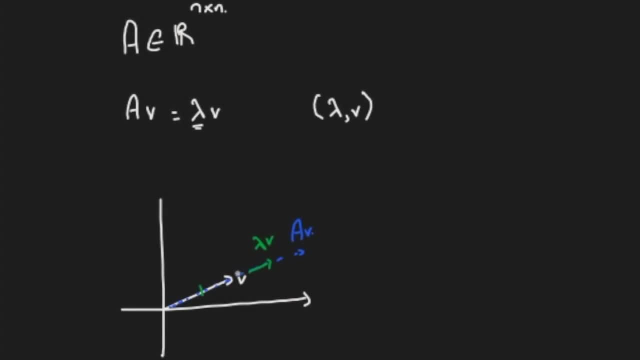 problems in numerical linear algebra. eigenvalues are critical in such fields as structural mechanics, nuclear physics, biology, the solution of differential equations, computer science, signal processing, electrical engineering, to name a few. eigenvalues also play a crucial role in the study of eigenvalues- vibrations, where they represent the natural modes or frequency of a system. 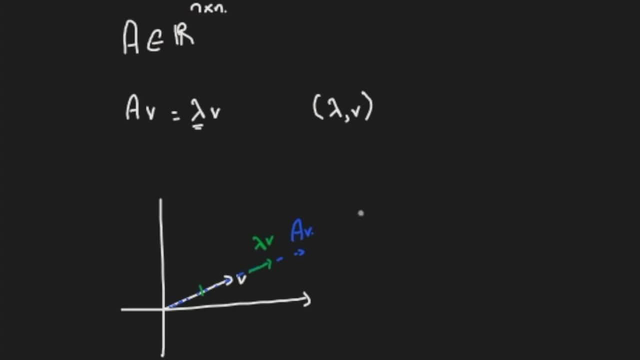 When vibrating structures begin to have larger and larger amplitudes of vibration, they can have colossal consequences. Some examples include the wobbling of the Millennium Bridge over the River Thames in London and the collapse of the Tacoma Narrows Bridge in the state of Washington. These are 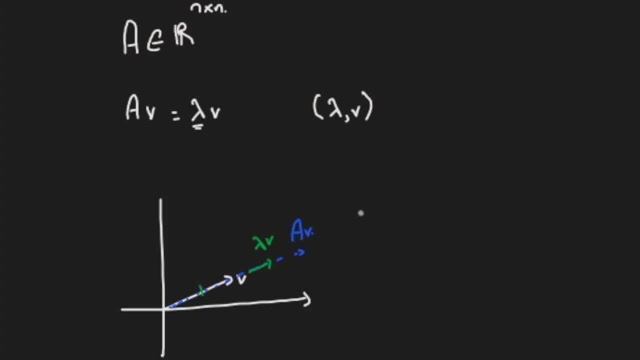 examples of a well-known phenomenon known as resonance. Now, a mathematical analysis of a general model for vibrating structures shows that when the system is excited by a harmonic force that depends on time, the system approaches a resonant state when the forces approach a particular eigenvalue. 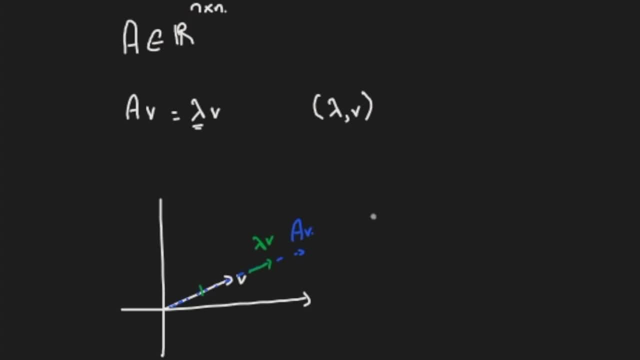 Now, later on in the course, we'll be giving applications, as we did previously with different concepts, such as encryption, when talking about determinants, or inverses, electrical circuits, when talking about linear systems, and trusses, as well, when talking about the same topic In a similar manner. 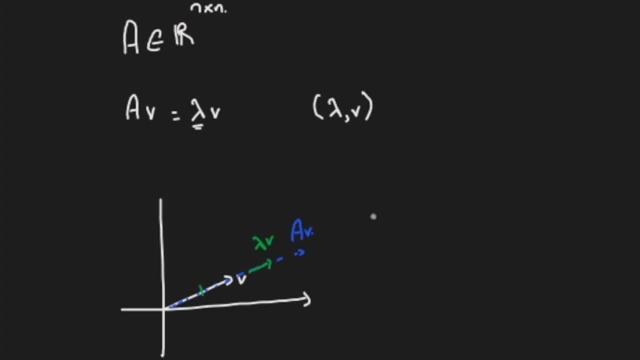 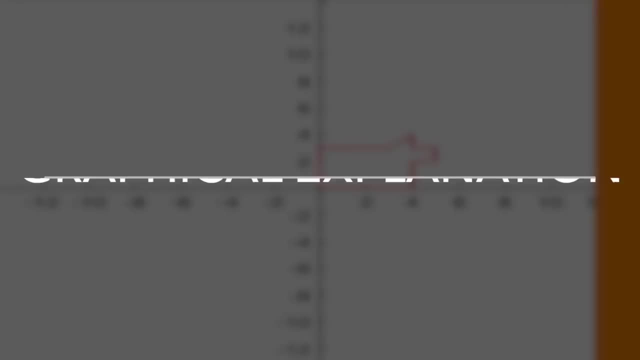 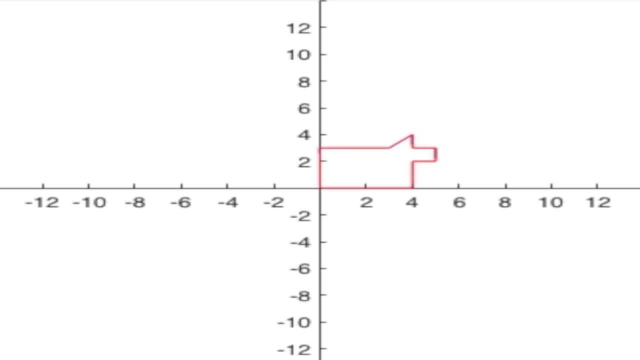 we're going to give applications to eigenvalues and eigenvectors to have a better intuitive feeling of what those quantities really reflect. Now do not forget that we're still talking about linear transformations, That is, we're going from one space to another via a linear transformation. So 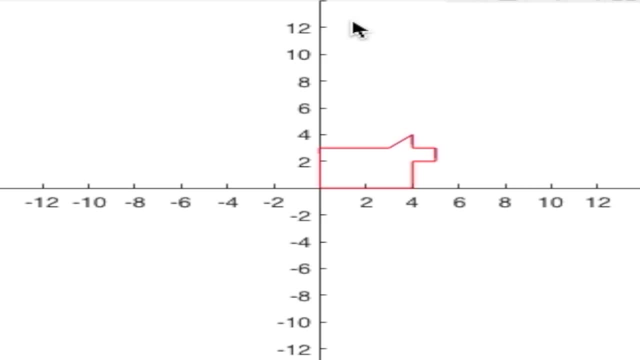 let's say we're in a 2x2 space and we're going from the traditional xy space to another space via this transformation matrix. So in this case it's identity, that is. any point, is brought back onto itself. Now, given the red shape over here, we'd 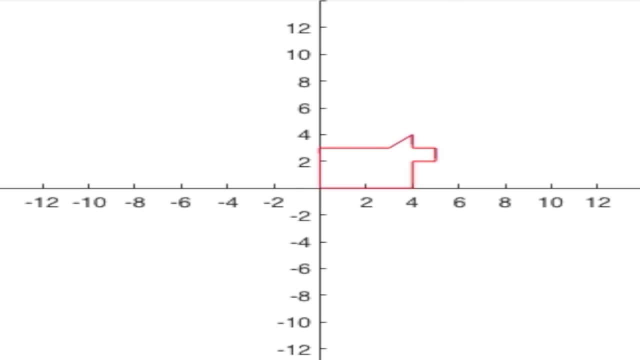 like to see how it's affected by different transformation matrices. So let's say, we're given this transformation matrix, Now the blue shape that looks like a horse is elongated along the x-axis, whereas it's preserved along the y-axis. Now, this is where eigenvalues and eigenvectors come. 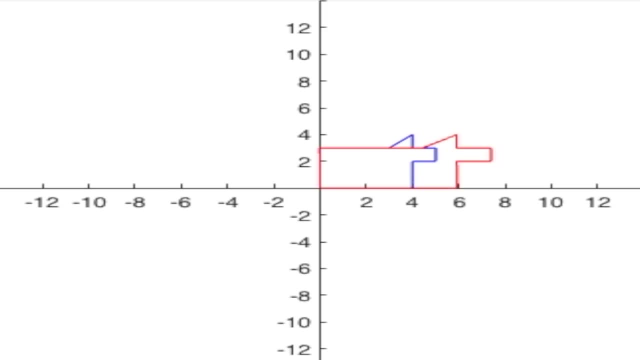 in hand. Why is that? Well, as you can see any point on this shape, let's say this point over here, that is, is brought to the point over here: 7.3 and 3, right, This tip right here, that is 4, 4 is brought to. 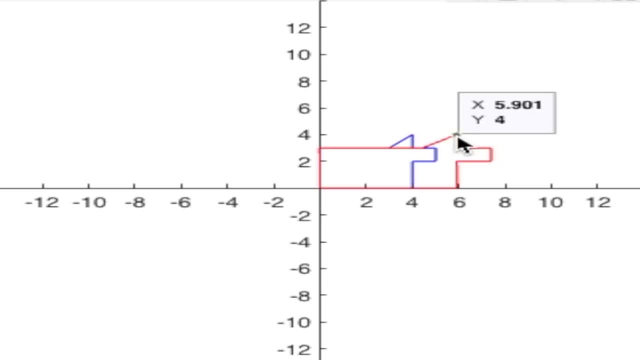 5.9, 4.. So what's going on here is that the magnitude along the y is preserved, whereas the magnitude along the x is amplified by 1.48.. It happens that one eigenvalue is 1.48 and its corresponding eigenvector is the unit vector. 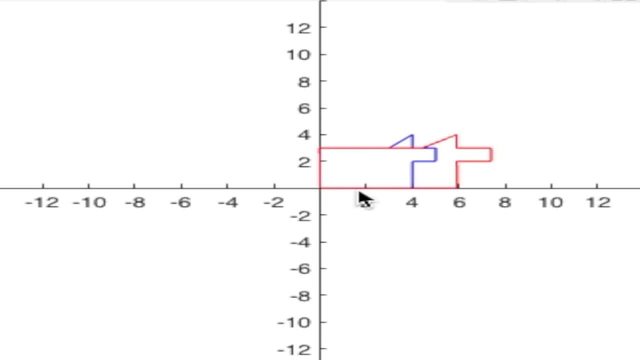 pointing towards the x-axis, That is 1: 0.. Why is that? Well, any point that is pointing along 1: 0, this vector over here, the x-axis, in other words, will remain on the x-axis after this transformation. So, as you can see, this line over here will just be. 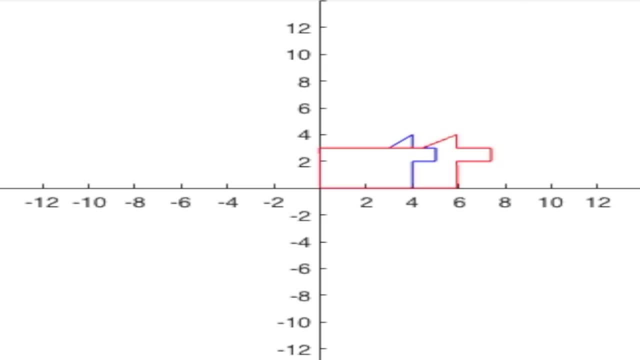 extended, It won't be shifted or rotated. Well, when does it rotate? Well, let's say we have this transformation. As you can see, the vector 1: 0 is no longer an eigenvector, The vector pointing towards the x-axis. well, it's no longer given. 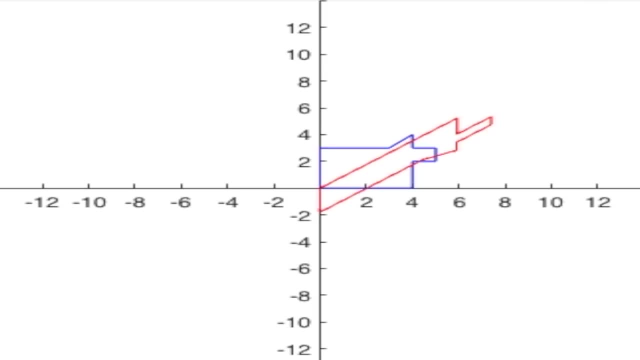 this other transformation. Other transformations could be, as such, shifting and rotating, rotating clockwise, compressing in one direction, and so on. So when thinking about eigenvalues and eigenvectors, it's, let's say, appreciated to keep the linear transformation concept in mind, because eigenvectors are specific directions. 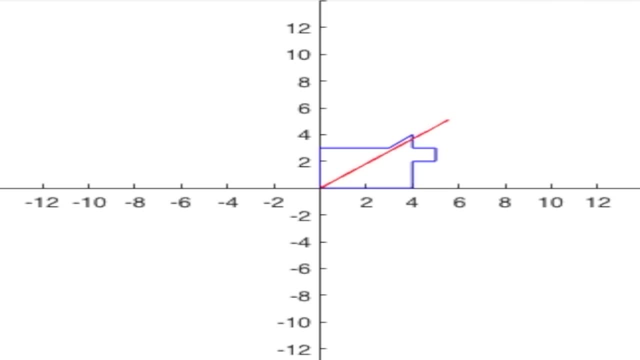 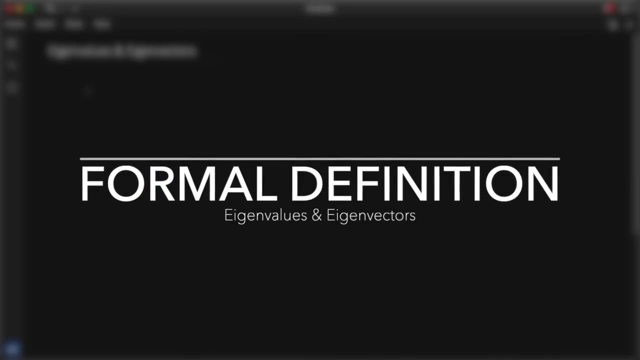 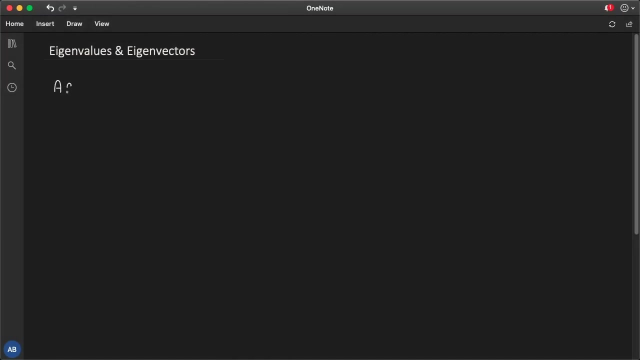 where the transformation is preserved, That is, the direction is kept unchanged. So let's get into a rigorous definition. So now to concretely define eigenvalues and eigenvectors. we'll start by a matrix A that is square And will always be square. There is no eigenvectors and eigenvalues defined for. 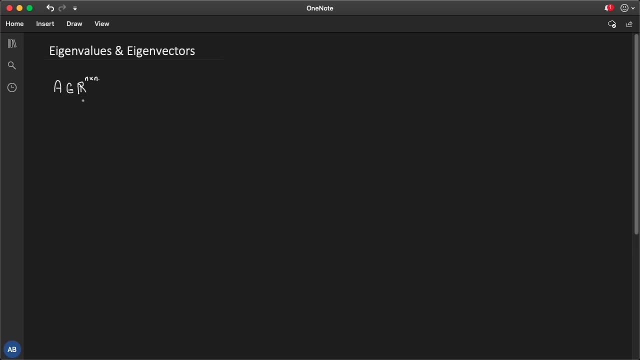 non-square matrices. Well, I'm not going to talk about this now, but there is a variation of eigenvalues, eigenvectors of this concept, towards non-square matrices, and it's called singular values and singular vectors. But we'll not talk about this in the few coming lectures. We'll postpone this to future lectures. 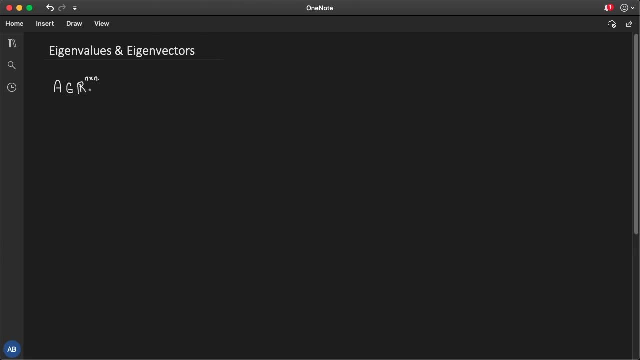 Now, in order to find an eigenvalue lambda and its associated eigenvector V, it must be the case that a V is lambda, V, right? If you're able to find me, simultaneously, a scalar lambda and a vector V that satisfy this equation, then guess what You found: an eigenvalue and its. 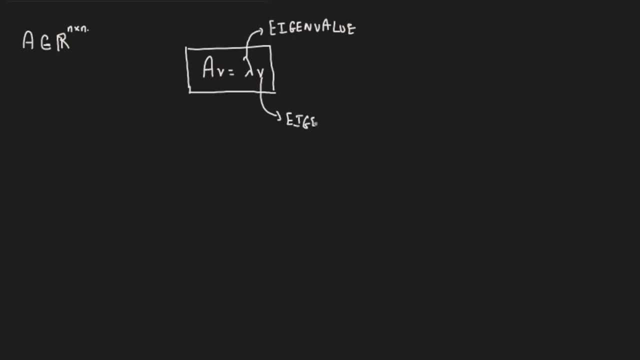 corresponding eigenvector right. Well, if we rewrite this equation well, we bring the right-hand side to the left-hand side, This is equivalent to a V minus lambda. V set to 0, the vector 0, right And factoring V, we get a minus, not lambda. many people do this mistake. it's. 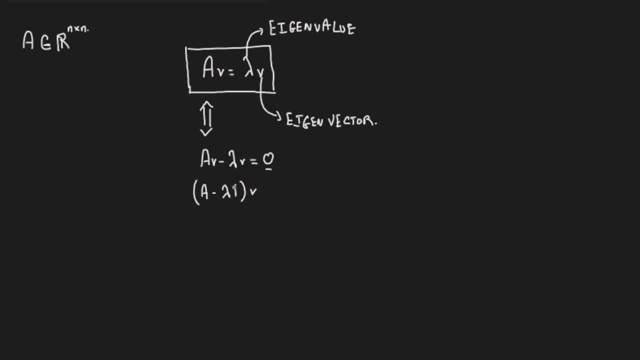 not lambda V. This is wrong. It should be lambda. I Okay The identity matrix I, because A minus lambda doesn't make sense. Actually, it's not defined. You've got a matrix, A minus a scalar. what does that mean? So 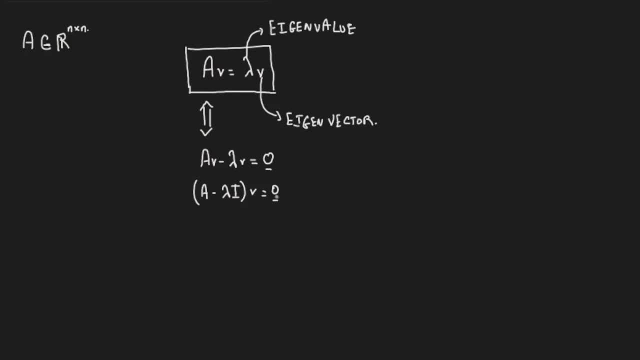 it's lambda, I? Okay. Now this is another way of rewriting eigenvalue relation, Since V is a nonzero vector. so we're not looking for the trivial solution to this linear system, we're looking for non-trivial solutions. Okay, And therefore, 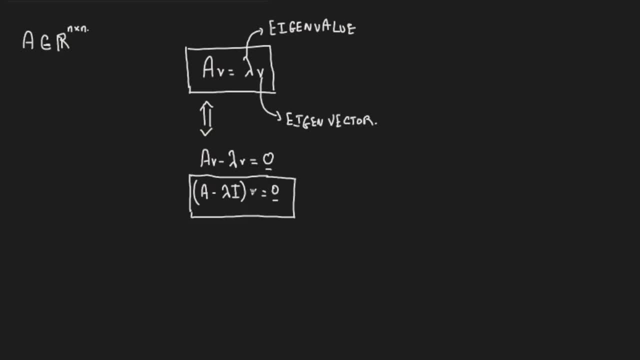 Because zero will always be. you know, an eigenvector. If I mean, look at it, What is a times zero? It's zero. Well, what is a lambda, such that lambda v is zero? It's anything. So there's infinite eigenvalues for the specific eigenvector zero. 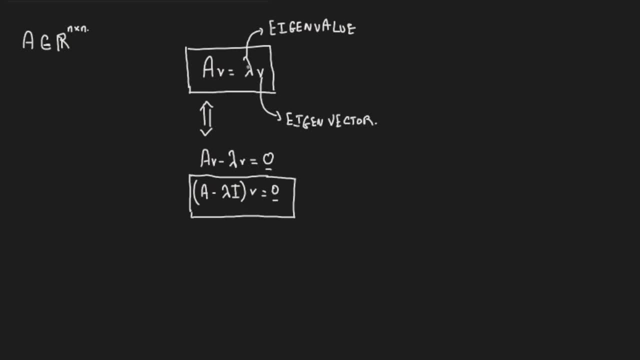 We don't care about this And we'll be only addressing non-zero eigenvectors. okay. Now what does that mean? It also means that the matrix A minus lambda I is singular. okay, So it is non-invertible. 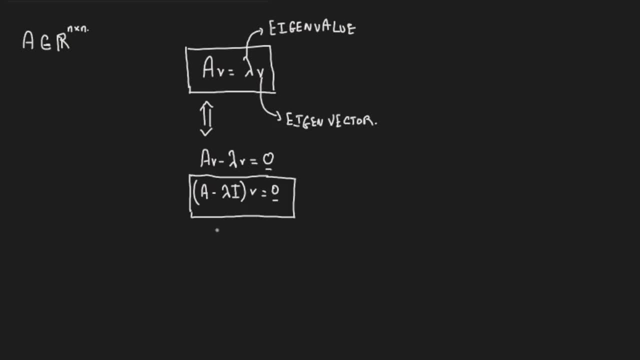 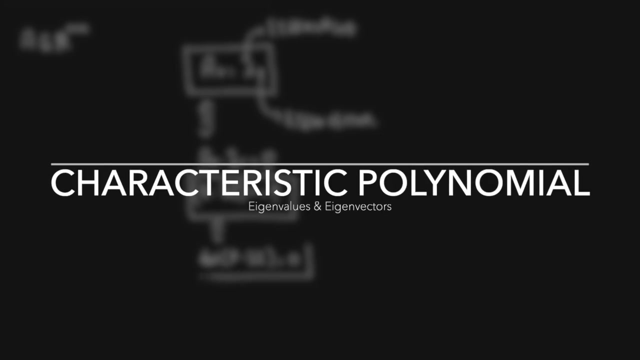 A minus lambda I, again, is non-invertible. What does that mean? It also means that the determinant of A minus lambda I is zero. This equation is very important And actually it has a name. So the determinant of A. 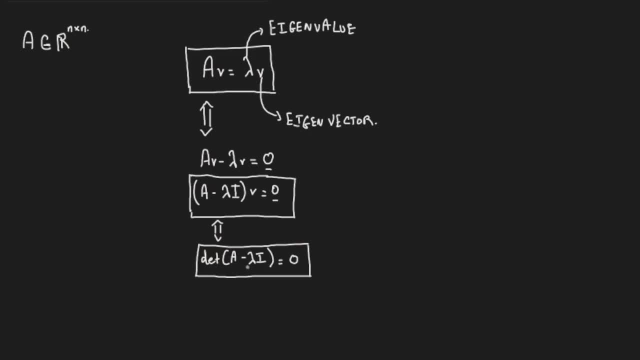 A minus lambda I is actually a polynomial of degree n, And the problem of finding the eigenvalues will boil down to finding roots or zeros of the polynomial determinant A minus lambda I. So why not see this determinant as a function of lambda, That is, P of lambda? 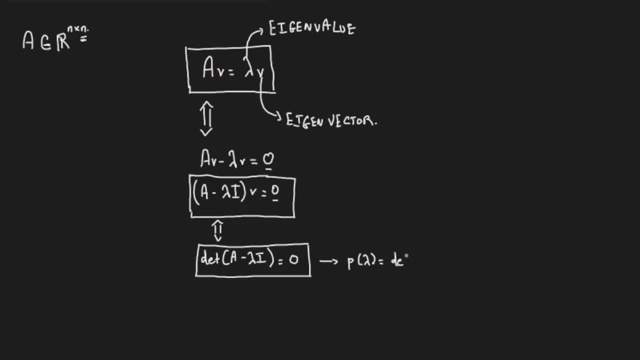 So P of lambda is actually the or is defined to be the determinant of A minus lambda I, And it is a polynomial, again, of degree n, That is we can write it as A n lambda to the power n plus A n minus 1 lambda to the power n minus 1. 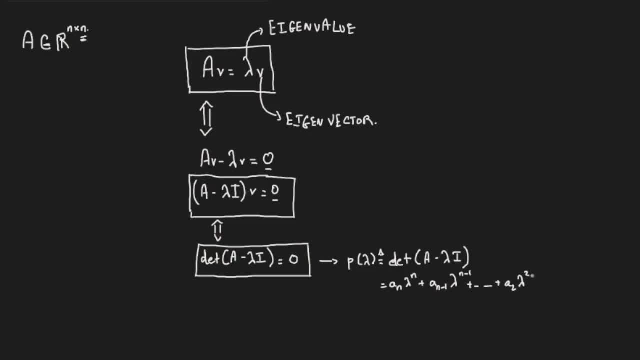 down to A 2 lambda squared plus A 1 lambda plus A 0.. And those A k's should not be confused with entries of matrix A. No, They are functions of the entries of matrix A, that's for sure. But they do not necessarily indicate entries. explicit entries of A. 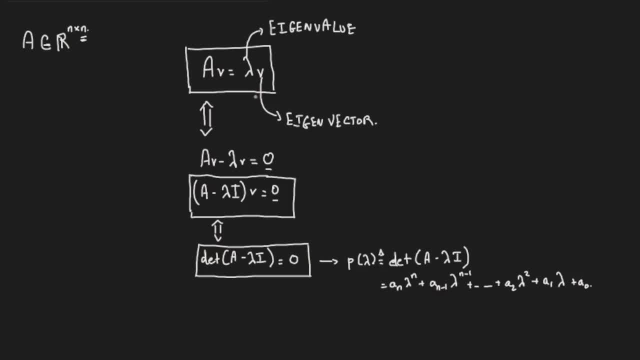 Okay. So keep in mind that I'm going to give you a small remark over here. Since P of lambda is of degree n, So the degree If P of lambda is n, this means that P of lambda. this applies in the real field. 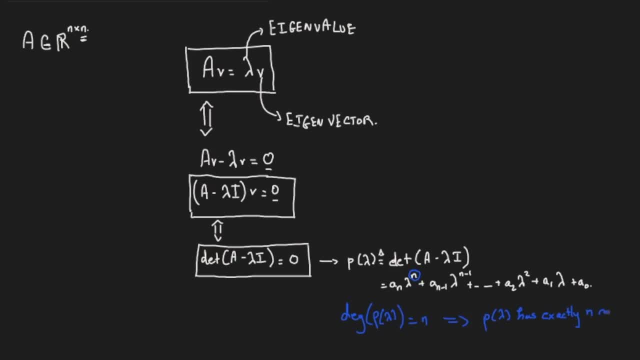 has exactly n roots or n zeros or n solutions, And any complex roots occur if the Well, this is our case When the coefficients are real: A, n, A n minus 1, down to A 2, A 1, A 0. 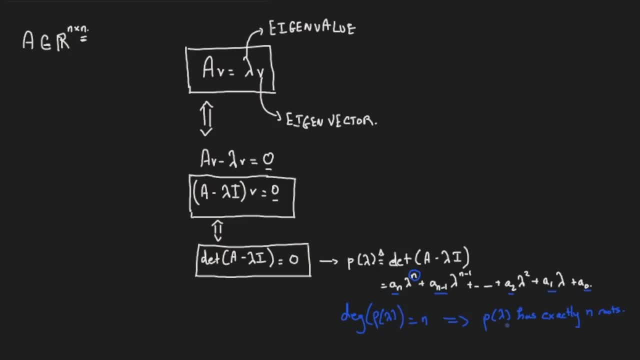 When those guys are real, which is our case, then in case you get complex roots, they appear. They appear in conjugate pairs. So an example on what I just said is the following polynomial: Imagine you've got a P of lambda, that is, I don't know, let's say lambda cubed plus 2 lambda squared. 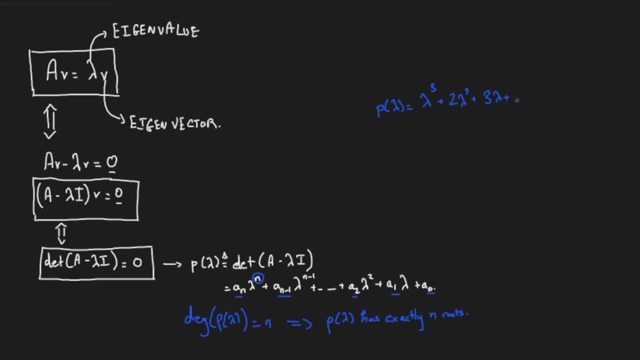 plus 3, lambda plus, I don't know, let's say 6.. Well, this polynomial, you can go ahead and verify that it has a real root. that is lambda 0, is- I don't know, that is lambda 0, equal to minus 2,. 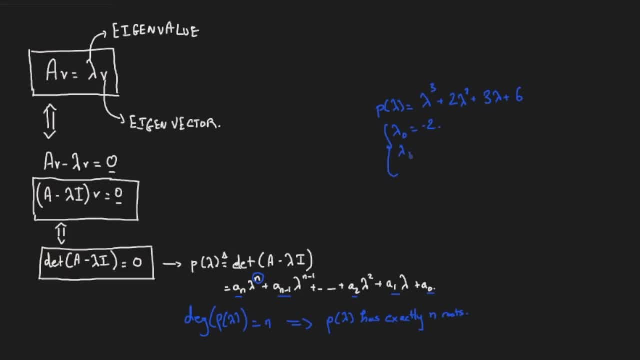 and two complex roots, lambda 1 and lambda 2, that are root 3i and minus root 3i. As you can see, they appear in conjugate pairs. Well, this doesn't only apply to this application. It applies to any polynomial with real coefficients. okay, 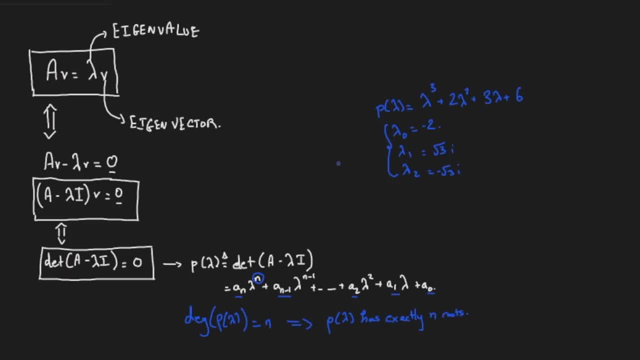 So this is always going to be our case for the next lectures, And the reason why is that A is a real matrix that will lead us to a polynomial P lambda with real coefficients And hence, in case we get complex roots, well, they appear in conjugate pairs. 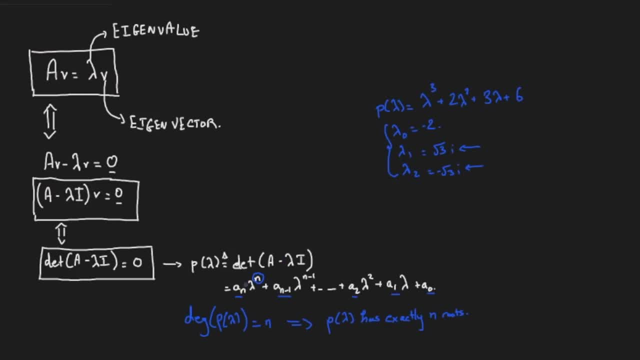 Now the polynomial. this polynomial of degree n may have one or more roots of multiplicity, or two or more. That said, you can encounter the following example. An easy, straightforward example is the following: Let's say P of lambda is lambda minus 3, cubed for example, or square. 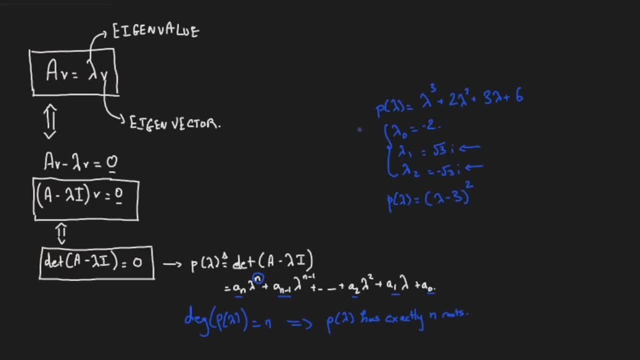 Let's keep it: lambda minus 3 squared. So this is example 1, and this is example 2.. This could be written as: lambda squared minus 6, lambda plus 9.. Well, what are the roots of P? They are lambda 0,, which is the same as lambda 1,, which is 3.. 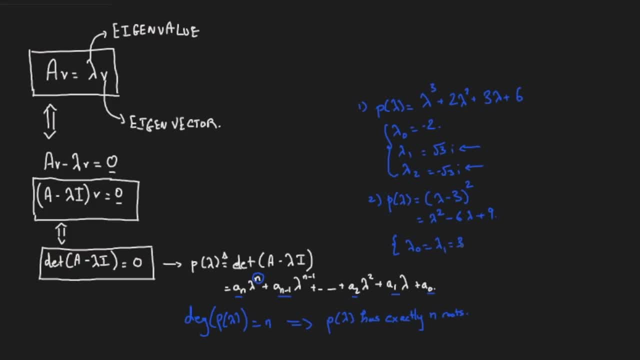 So we got two roots that are equal. We say that this root 3 is of multiplicity 2. That is, it appears twice. We also say that the root 3 is counted two times or twice. okay, Now keep in mind one thing. 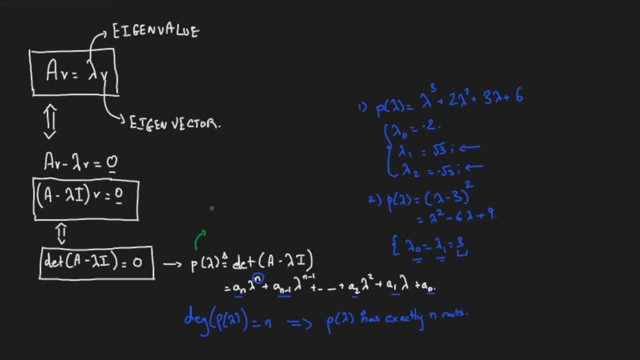 This polynomial P is called the character characteristic equation of matrix A. okay, Now I know I've said a lot of stuff over here, but it's really, it's really worthy to rewrite the eigenvalue relation in different ways, because this relation led us to this. 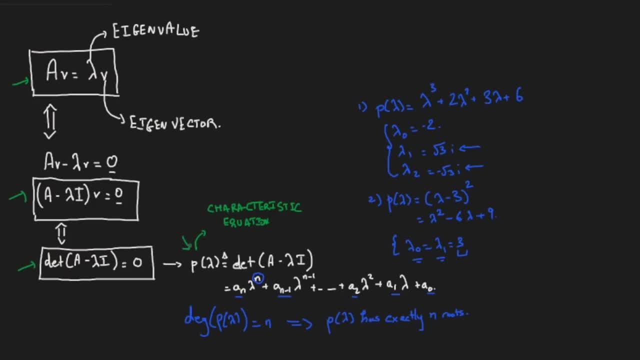 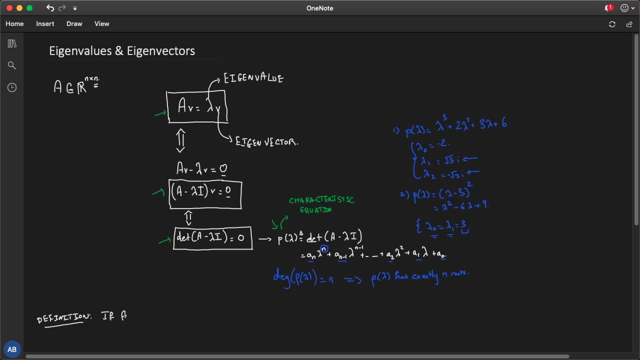 which led us to this and, finally, to this very important polynomial, because really this is how we're going to find the eigenvalues. This is the classical way of detecting the eigenvalues. So, more formally, if A is a real square matrix, 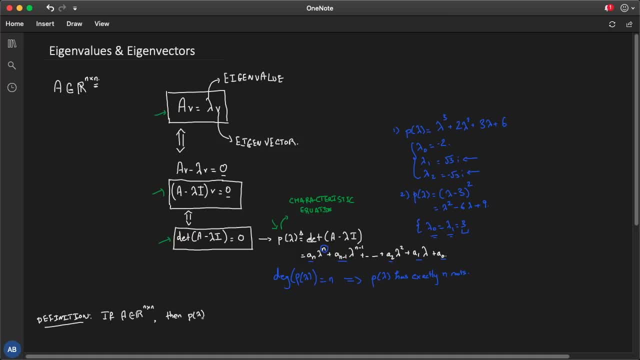 then the polynomial P lambda that is defined as determinant of A minus lambda I is called the characteristic polynomial. Actually this equation over here it should be replaced by polynomial. The term equation is when you set the characteristic polynomial to zero. so P lambda equals zero is called the. 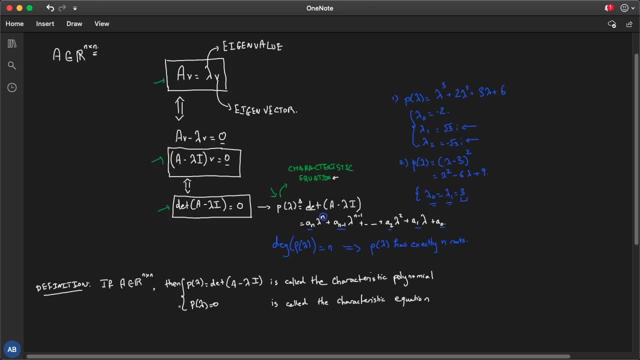 characteristic equation. okay. So again, why do we care about P of lambda? Well, if a particular lambda call it lambda naught is a root of P of lambda, that is, P of lambda naught is zero, then lambda zero is an eigenvalue of matrix A. 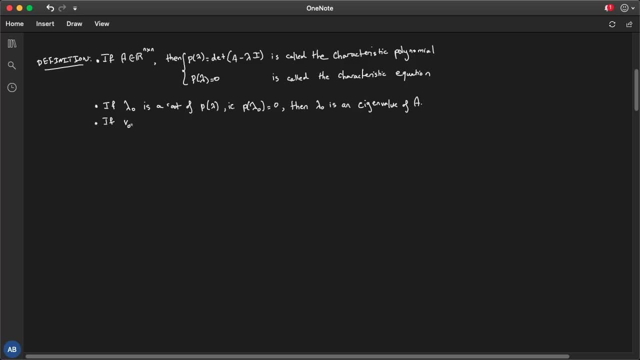 And even more. if vector V zero is a non-zero column vector, satisfying a V zero is lambda zero V zero, then V zero is an eigenvector of A. okay, So this is what we're going to do. So we're going to do this. 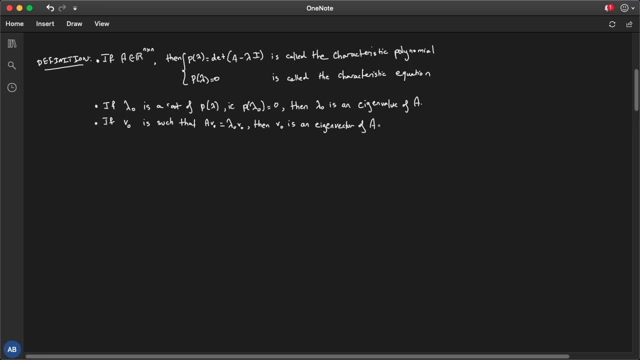 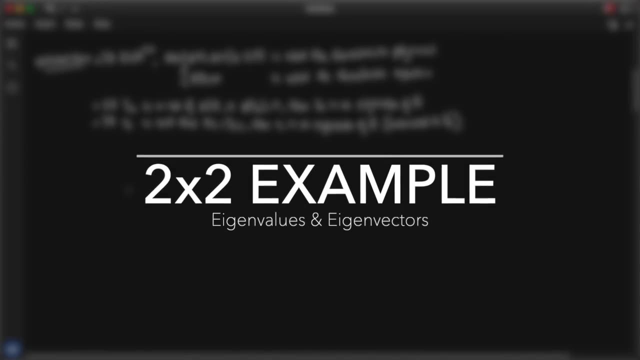 So we're going to do this. So we're going to do this. Let's draw that line. So let's say that vector V zero is F of A And it is, you know, associated to lambda zero. So let's give an example on eigenvalues, eigenvectors: 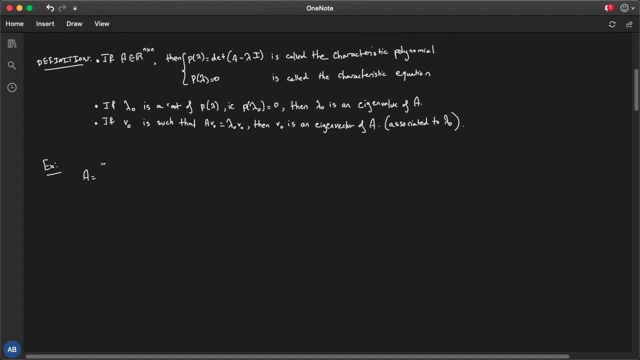 So an example on this would be: Say we've got a matrix, Let's say 2, 1, and 1, 2, okay, And you're asked to. And let's say we're given two vectors, V, zero. 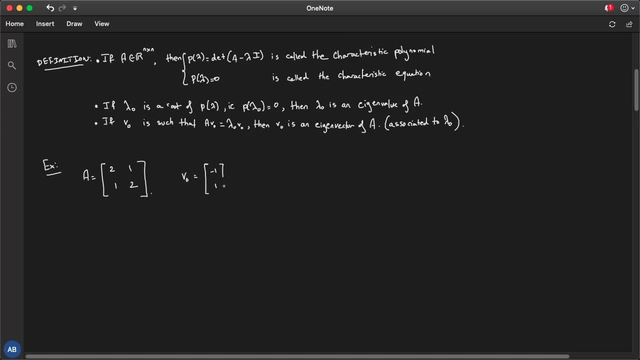 That is minus one one and v one. that is one one, and we're curious to know if any of the two vectors are indeed our eigenvectors or not, what? what we have to do is just to see if is a v a scalar multiple of v. that's what you have to ask yourself. well, we start with a v zero. 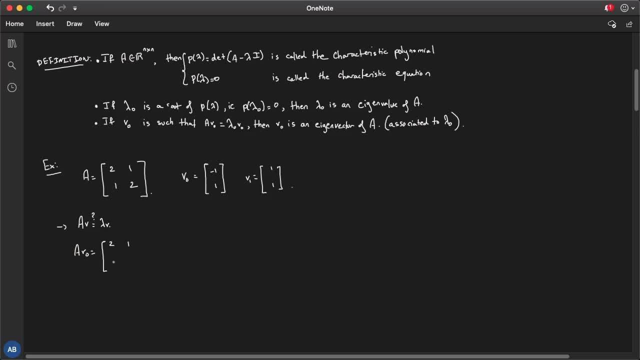 that is two, one one, two by minus one and one. that gives us minus one and one. so it didn't only give me lambda v zero, it returned v zero as is. so what do we say? we say that v zero is, is an eigenvector with. 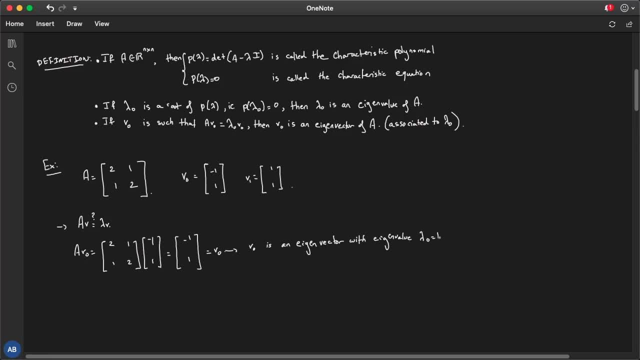 eigenvalue lambda zero is one. now let's check v one. so a v one is following product, that is three, three. now is this a scalar multiple of v one? well, yes, why? because you can write it as three times one. one, that is three v one. so we say that: 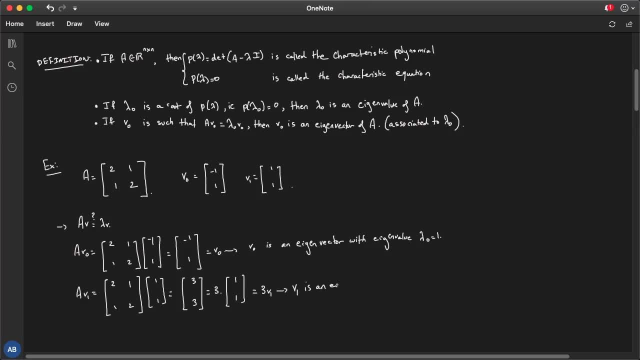 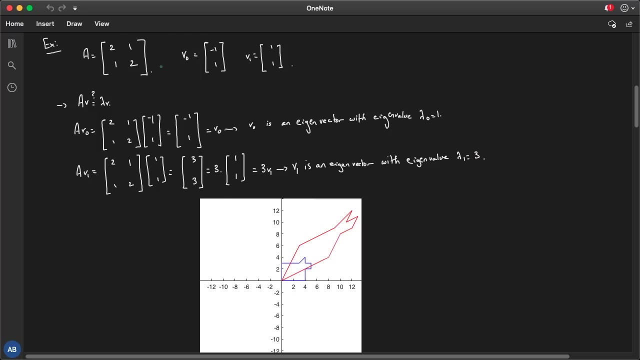 v. one is also an eigenvector with eigenvalue lambda. one is three right, right. so back to the horse example. let's say my transformation matrix. is this guy right? and we would like to visualize how eigenvalues come in place. well, the first eigenvector is not going to be the first one. 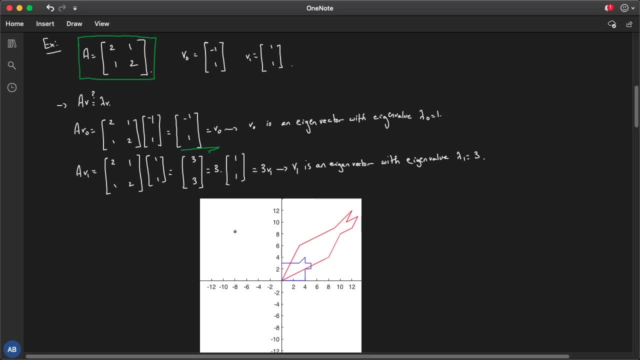 to really be of interest over here, and that's because it's pointing towards minus one and one. so something like this right um v one, on the other hand, is going to be an eigenvector of interest. why? because we've got a point over here pointing in its direction. 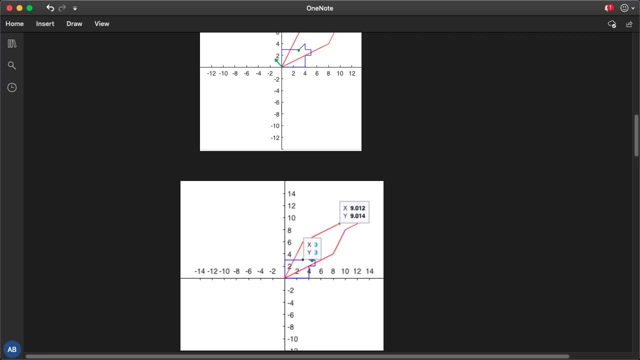 that is three, three. it lies on the, on the square of the analysis, where the action vector is pointing to the even vector, with value i equal to negative 3.3, and what that means is: if v. so if this is going to give us one trademark, that's going to be ours in this equation, yeah, we go down into the cut-off suits of the fixed component, which, in that case, v is positive. v is divided by three, which is minus 1 ft, which is positive. v is equal to 하나 square, that which means there is only one other. 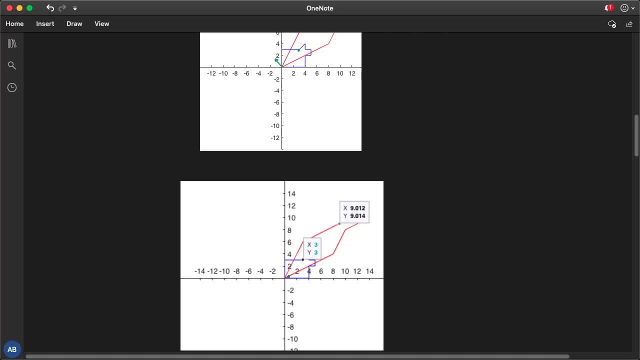 on the line that is in the direction of one one Right. So, that said, this point over here will be transformed to the point on the same line, right, And even more, since the eigenvalue is three. then guess what? 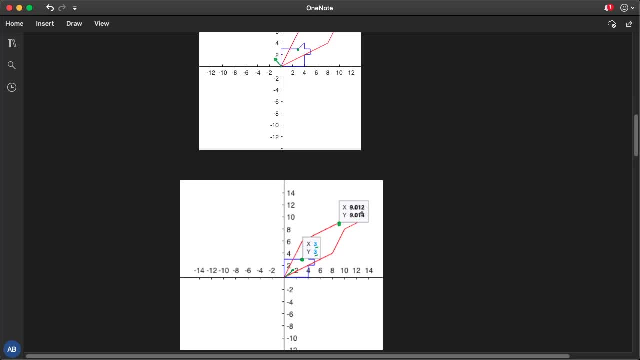 Those points over here will be multiplied by three, And just forget the decimal notation for now. It's just that I didn't manage to get the point on the exact point. I got it somewhere next to it. Well, it should be nine by nine. 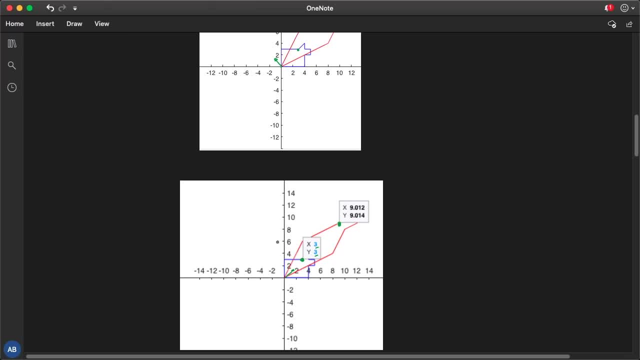 So the point that we transformed is not rotating, is not doing anything other than being amplified on the same direction. So three, three becomes a nine, nine, And that's what eigenvectors, eigenvalue and eigenvalue Reflect. After transformation, the point preserves direction. 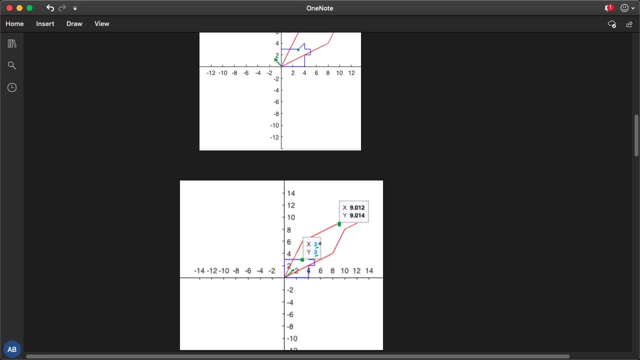 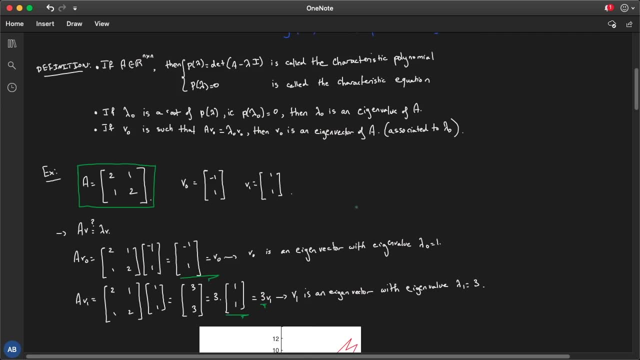 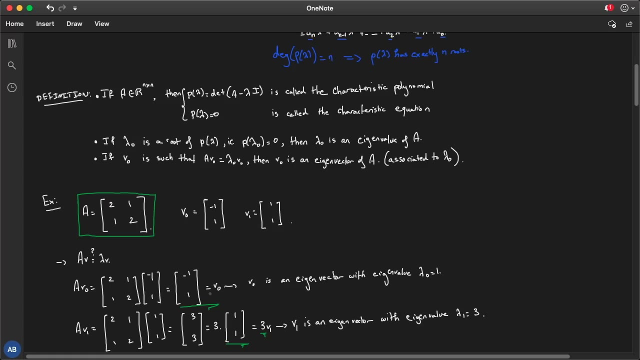 and is either elongated or compressed. In this case it's elongated because the eigenvalue three is greater than one. Okay, So in this case we got a multiplicity of one per eigenvalue. So one showed in ones and minus one. 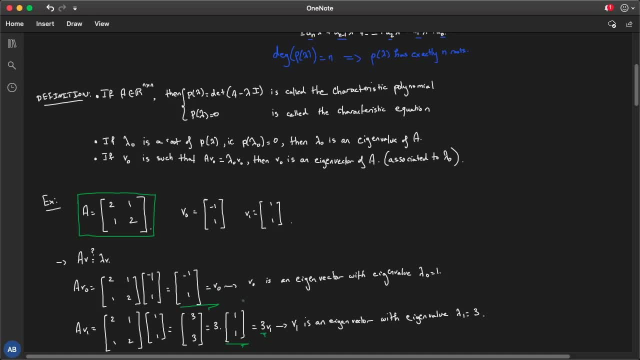 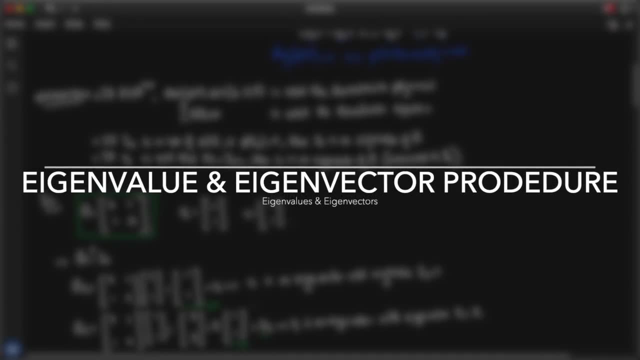 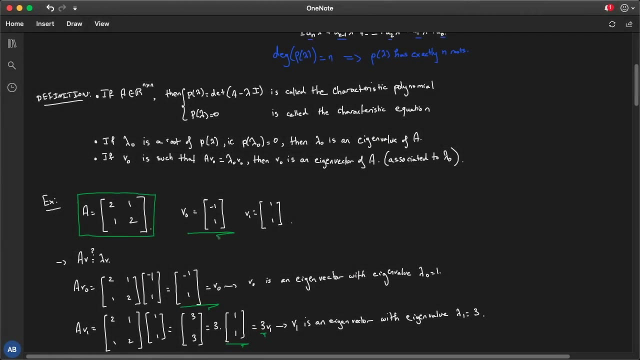 and three showed in ones We didn't see and I can value with two eigenvectors, even though this is possible. Now, let's say we want a procedure to find eigenvalues and eigenvectors When here, in this example, I gave you two vectors and I told you to test. 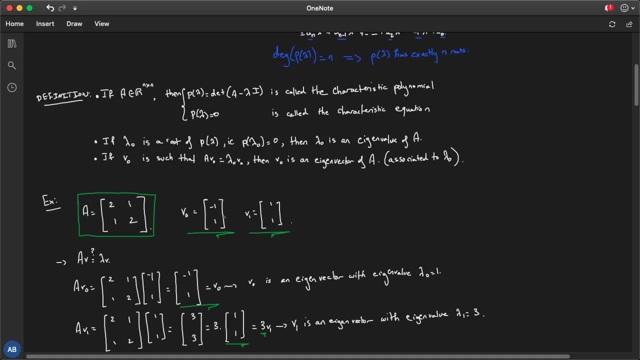 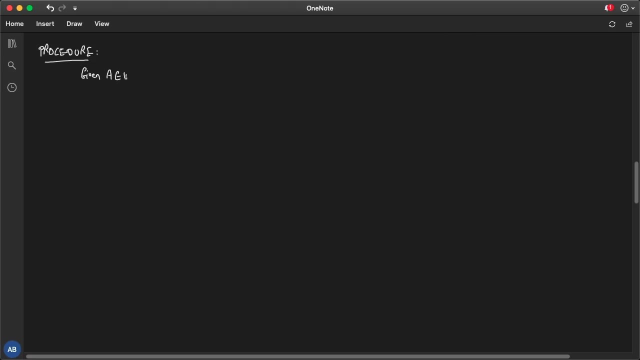 if those factors are indeed eigenvectors or not. Well, let's say, I'm only given the matrix A without the eigenvectors V zero and V one. Well, there is a procedure for that, And the way of doing so is: given A is N by N. 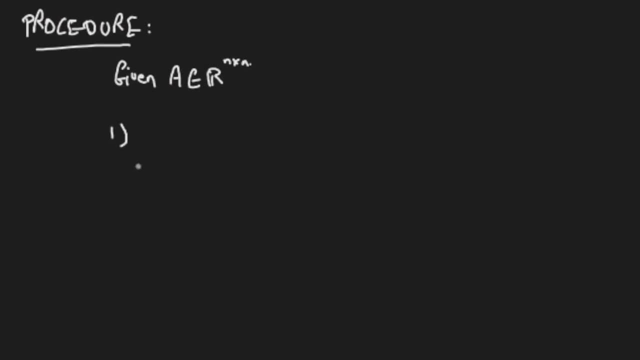 How do we proceed? So, one, we find the characteristic polynomial P of Lambda that is defined by the determinant of A minus Lambda I. Two, we compute using what you know in calculus. really, Really this is not really sophisticated, So compute. 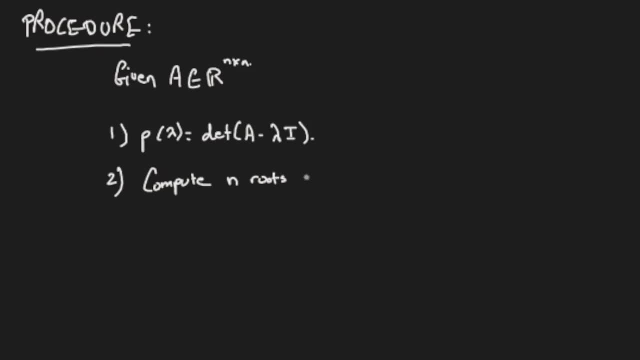 N roots of the characteristic equation. P of Lambda is zero, right. The roots are labeled by Lambda one down to Lambda N. So N roots, Those are the eigenvalues of A, Now three for each distinct Lambda I. so we find vectors such that 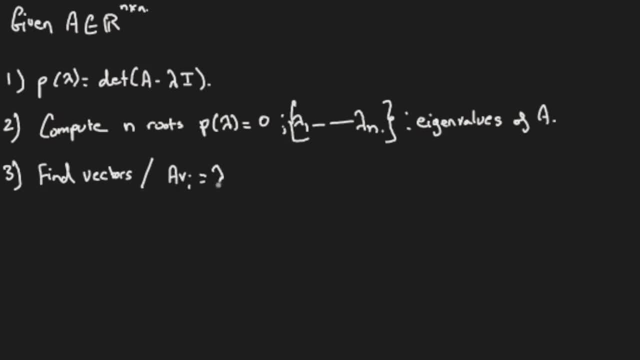 A V I is Lambda I V I By. you know you can do this however you want, but usually what people do is solve A minus Lambda I V I is zero. Solve this homogeneous system Now, in case Lambda I is of multiple roots. 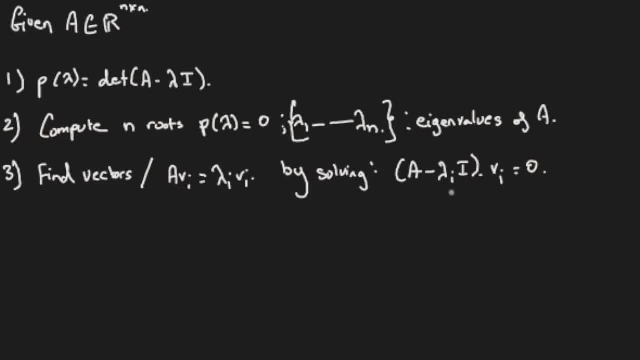 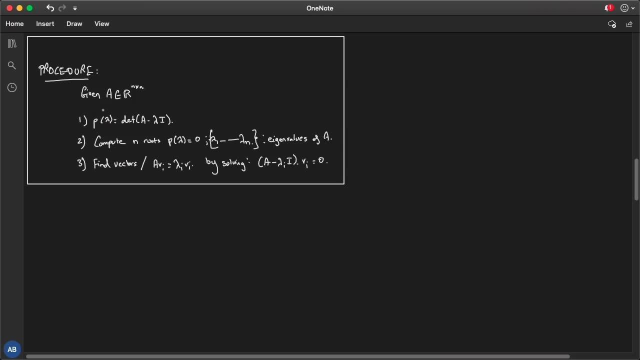 we'll see this later on. there may be only one associated eigenvector, If not just compute the distinct eigenvectors. Okay, So this is the procedure. This is how you do it. So let's do an example, taking the same matrix A. 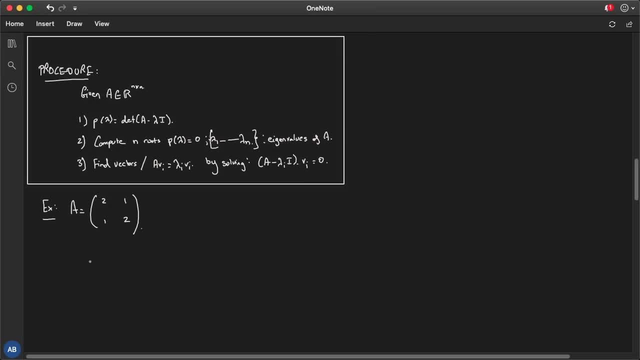 that is two, one, one, two, and try to figure out, without any given vectors, the eigenvalues and eigenvectors of A. So applying this procedure, first compute the characteristic polynomial P of Lambda, That is the determinant of A minus Lambda I. 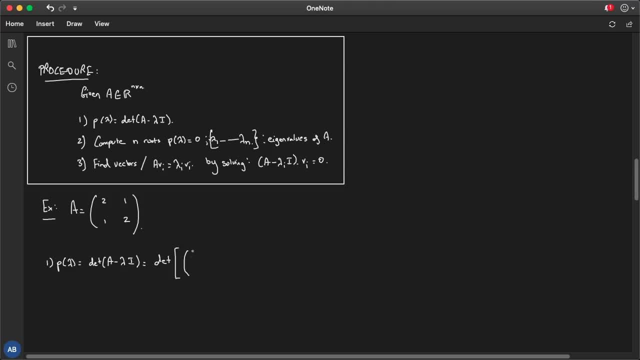 That is the determinant of A, that is two. one. one two and Lambda. I is always an identity with Lambda on its diagonal components, right? So doing the math, we get the determinant of two minus Lambda here. one minus zero, that is one, one minus zero. 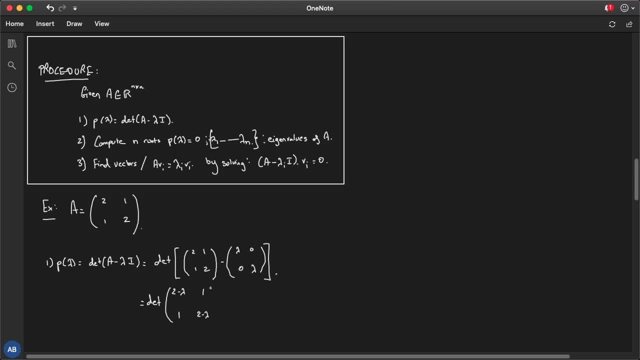 that is one and two minus Lambda. again The determinant. we do this cross thing to get two minus Lambda times two minus Lambda, that is two minus Lambda square minus one times one, that is one. right. You could also write this as Lambda minus two square. 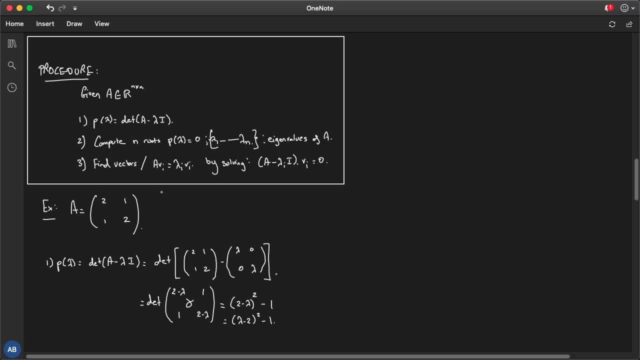 minus one. Now here to go to step two. you want to find the roots. Well, from calculus, from what you know, in calculus find finding roots of polynomials are easily done when the polynomial is factored, So using really an identity here. 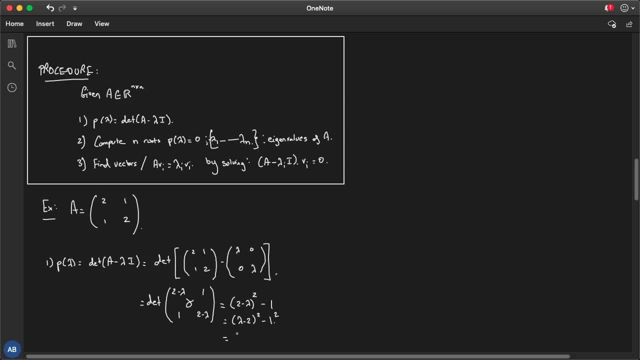 that is A square minus B. square is A minus B into A plus B. So we get Lambda minus two minus one into Lambda minus two plus one. right, That is Lambda minus three times Lambda minus one. Now writing down the characteristic equation: 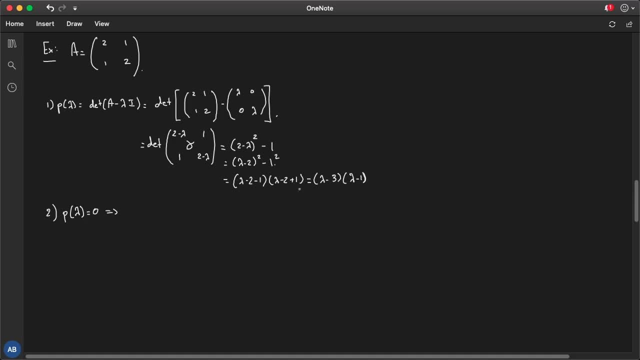 P of Lambda equals zero. we grab the factored form of P of Lambda, that is, Lambda minus three, into Lambda minus one, that is zero. This is the equivalent of saying Lambda one is three. So the roots are: Lambda one is three and Lambda two is one. 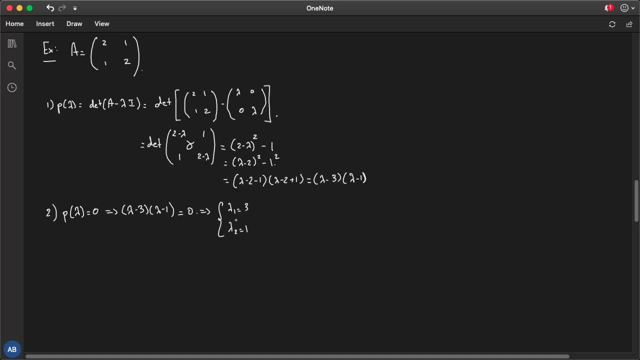 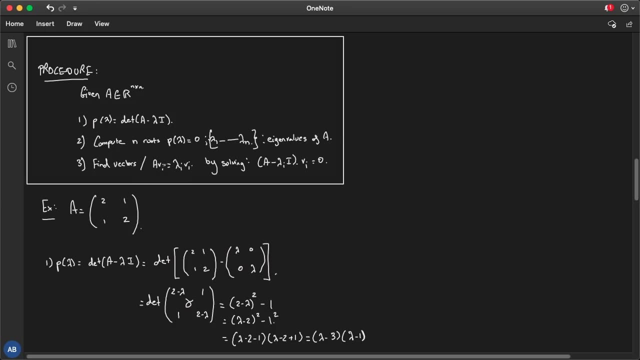 So we successfully got the eigenvalues of A, that are three and one. Going down to the last step, that is, for each Lambda I, we find a vector VI that satisfies the eigenvalue relation, either by solving this or this. So, doing this, here, let's grab Lambda one equal three. first, 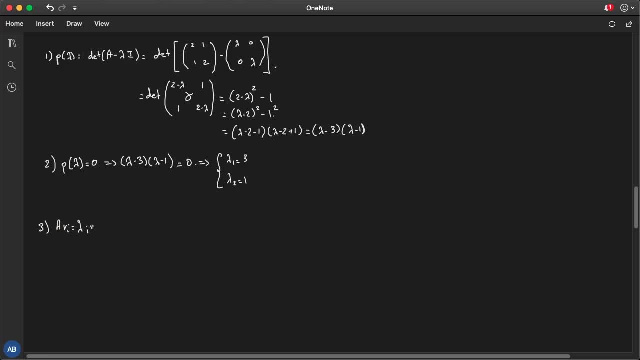 So A VI is Lambda I VI. So for Lambda one equal three. we want to find V one such that a V one is three V one. right Now we replace: A is two, one one two V one is unknown. 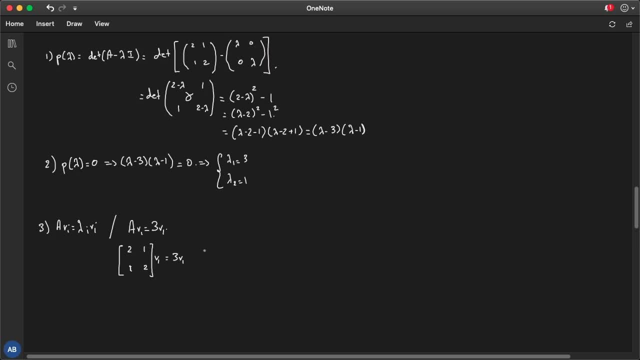 We're trying to find it. This is three V one. Now, if you denote by V one a vector of unknown components, let's say X and Y, the problem is to find your X and Y right. So two, one one, two multiplied by a vector of XY. 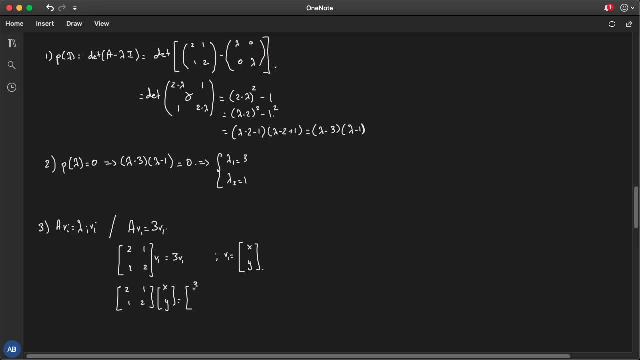 is nothing other than three X and three Y. right Doing the math, what you get is two X plus Y, the first component, and X plus two Y in the second one. That is equal to, again, three X and three Y. 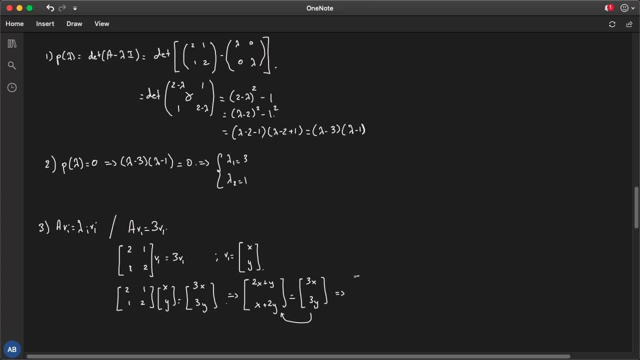 Well, if we get this vector on the left-hand side, what we get is minus X plus Y. So let's start from the left-hand side. minus X plus Y and X minus Y- right, That are both equal to zero. 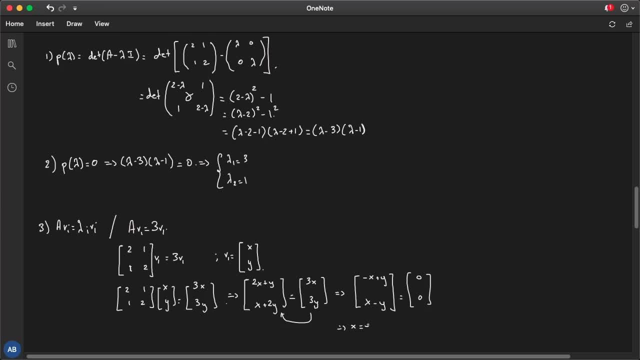 Well, both equations are giving us that X is equal to Y And for that you can pick: Y is equal to one. to get X one. Okay, Actually, if you notice, you can pick any Y, you can pick a two so that it's corresponding: X is two. 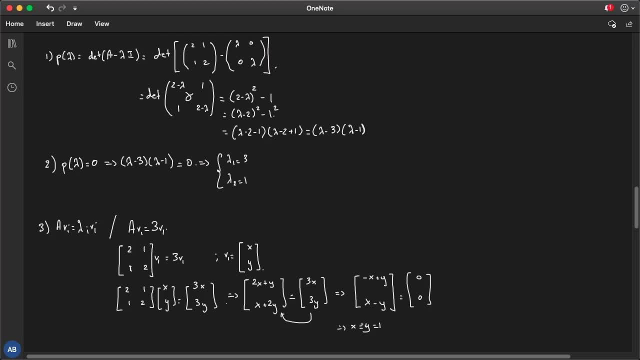 You can pick a Y three, because really here what we care about is the direction. So a direction in the one, one sense, it's what we care about. a unit direction. Okay, So one eigenvector V one is one one. 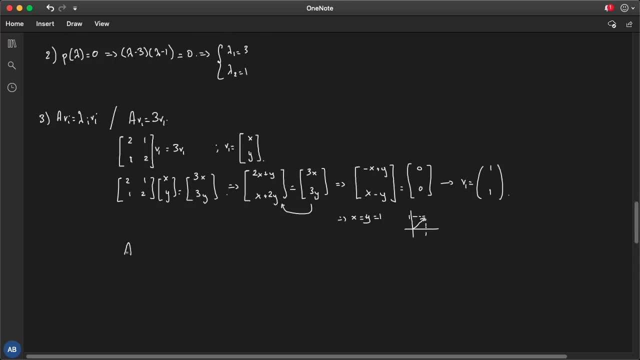 Now doing the same thing for the second eigenvalue: a V two is Lambda two, V two where Lambda two is one. So a V two is one, A V two is V two, And again the denoting V two by X, Y. 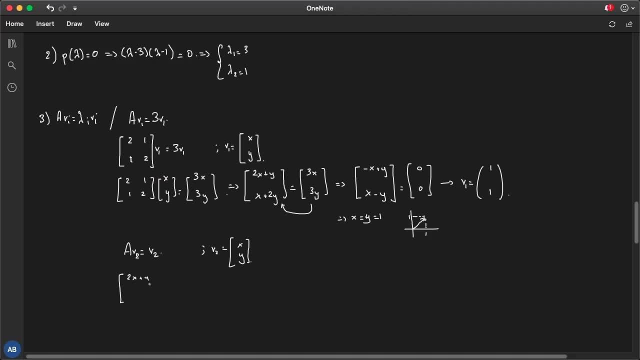 performing the multiplication, we get two X plus Y, and X plus two Y is equal to X- Y, right? Getting this guy over here. we got X plus Y and also X plus Y. that is zero, zero. So we get X is minus Y, right? 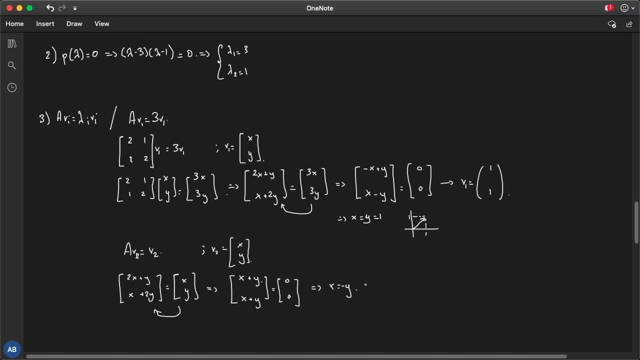 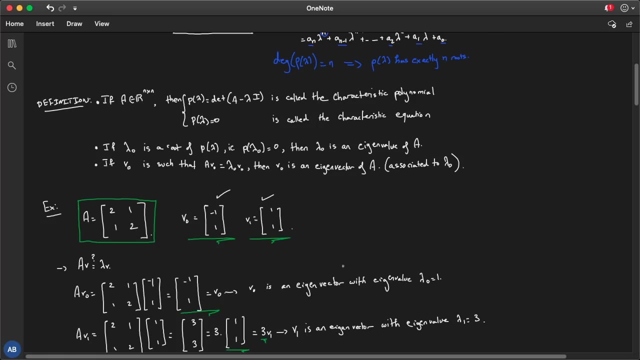 You can pick Y to be one, so that your X is minus one. So V two is one minus one, or even minus one one. right Going back up here we get the same results. Lambda one: here is one. Now I didn't do the numbering correctly. 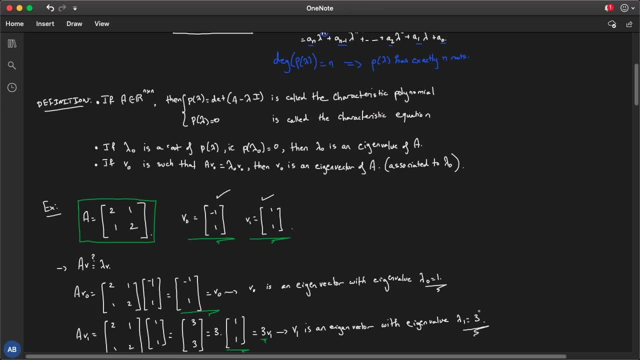 but that doesn't matter. All what matters is: an eigenvalue is matched with its suitable eigenvector, So three is matched. So the eigenvector one, one and one is matched with this eigenvector minus one, one. Okay, 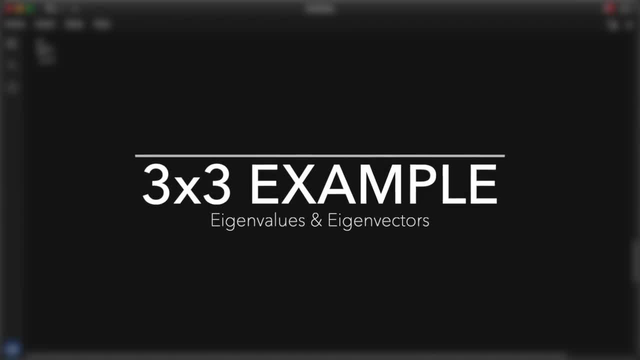 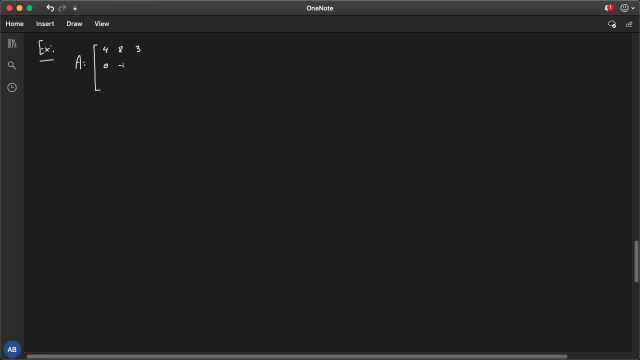 Now let's see some more interesting examples. Let's say I've got the following: three by three, matrix A, that is four, eight, three, zero minus one zero and zero minus two and two. Let's compute the characteristic polynomial That is determinant of A minus Lambda I. 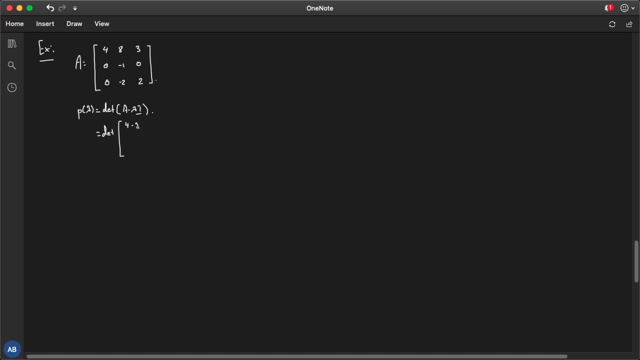 Which is the determinant of four minus Lambda, eight, three zero minus one minus Lambda and zero, zero minus two and two minus Lambda. Well, since this column is all zeros except the first component, so we'll compute the determinant based on that. 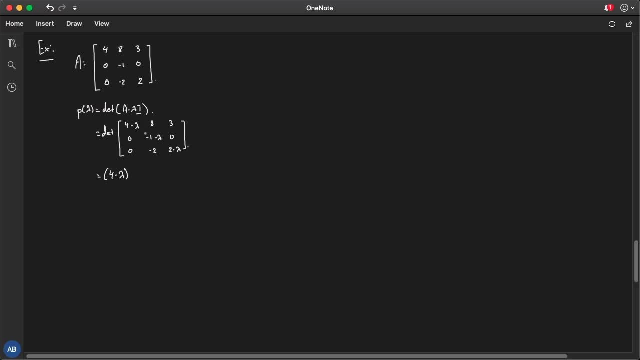 And hence we'll get four minus Lambda times the determinant of this matrix over here. right, That is minus one minus Lambda into two minus Lambda minus zero times minus two. So this is what we get, And hence computing the eigenvalues is as simple. 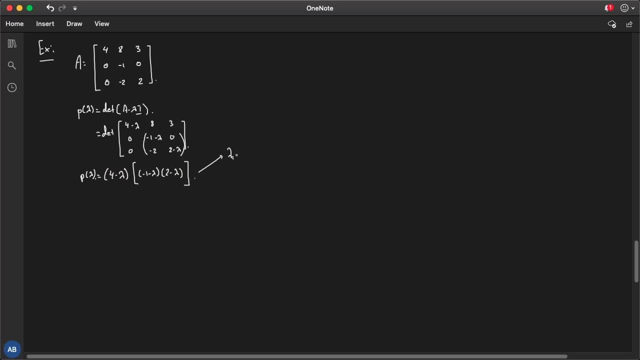 as finding the roots of this polynomial, We get: Lambda one is four from this factor, Lambda two is minus one from this factor And Lambda three is two from this factor. So now we found the eigenvalues, So let's find the eigenvectors. 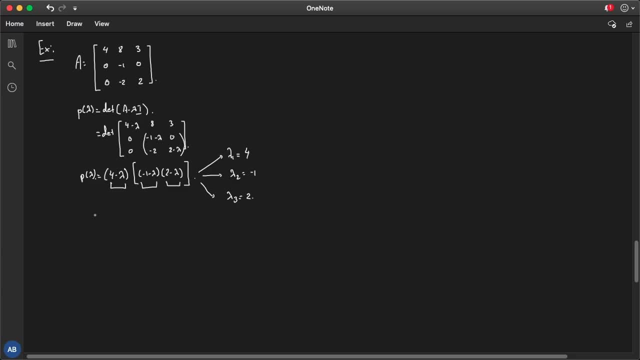 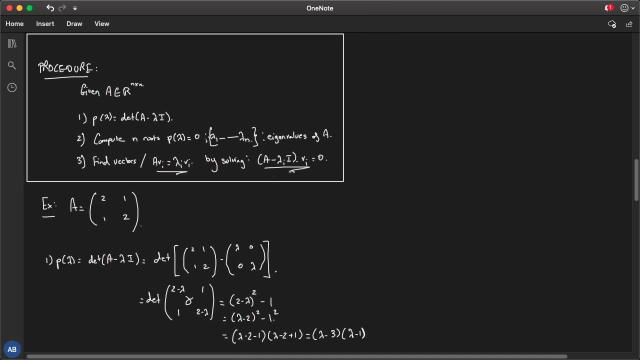 Okay. So in this example, instead of you know, solving for A VI is Lambda I VI. we're going to use the other form, That is, the one over here. Okay, A minus Lambda I times the I all multiplied by VI is zero. 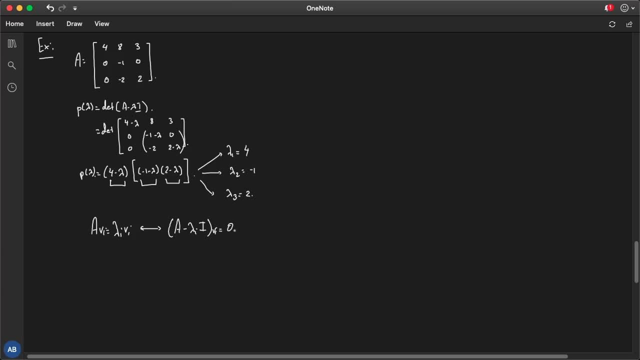 So instead of this, we'll be using this. So what is A minus Lambda I times the I. Actually, what is A minus Lambda I? It's this form over here, So writing it down over here: four minus Lambda. eight and three: zero minus one minus Lambda. 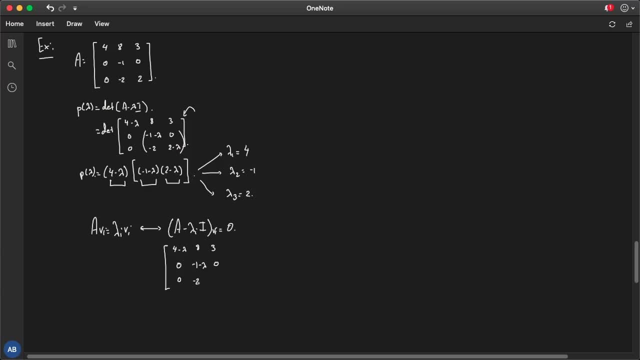 multiplied by zero, zero minus two and two minus Lambda, all multiplied by a vector VI of components X, Y and Z is the vector of zeros. right Now we've got three vectors of this form that we need to find: V1, that is linked to Lambda one. 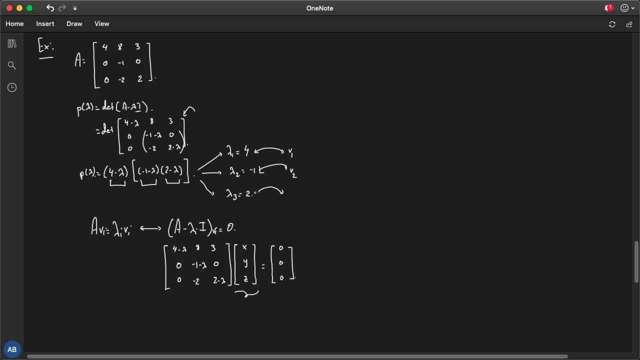 V2 associated to Lambda two, and likewise V3 associated to Lambda three. So this is the A minus Lambda I. So at Lambda I equal to four. So for Lambda one, what do we get? So all you have to do is replace Lambda I. 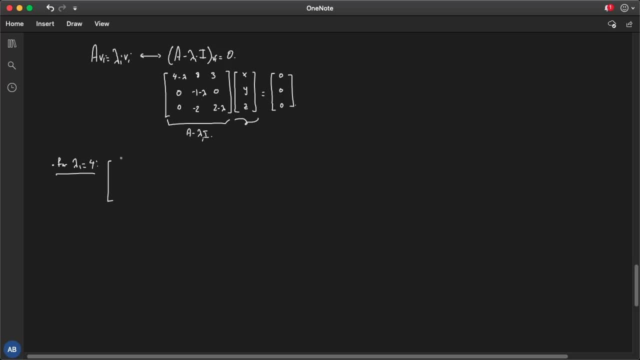 replace Lambda with four and then compute. So four minus four is zero. Then the rest are unchanged. Minus one minus four is minus five, and two minus four is minus two. So this is a homogeneous system that we can easily solve through Gaussian elimination. 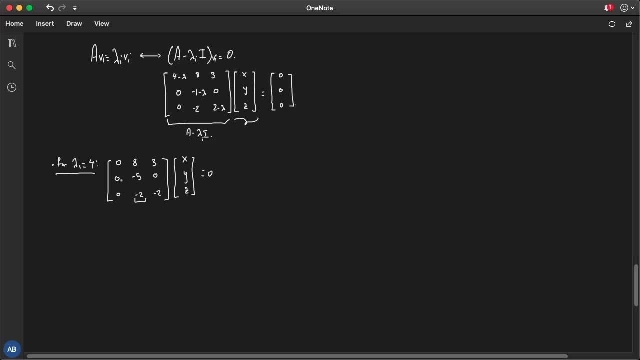 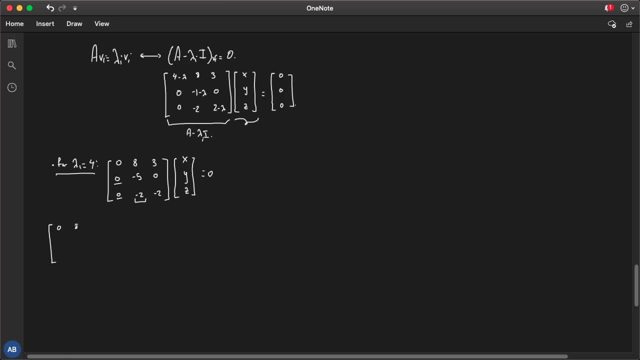 All we have to do is write this down here and perform one step of Gaussian elimination. That is, instead of R3, we put in R3 minus two over five R2, right, What do we get? The first two rows are unchanged. 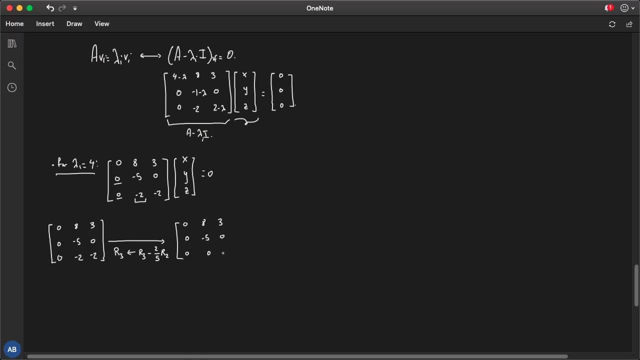 whereas the last one becomes zero, zero and minus two. right, So we're still solving. Do not forget the important property of this. Do not forget the important property of this. Do not forget the important property of this. Do not forget the important property of Gaussian elimination. 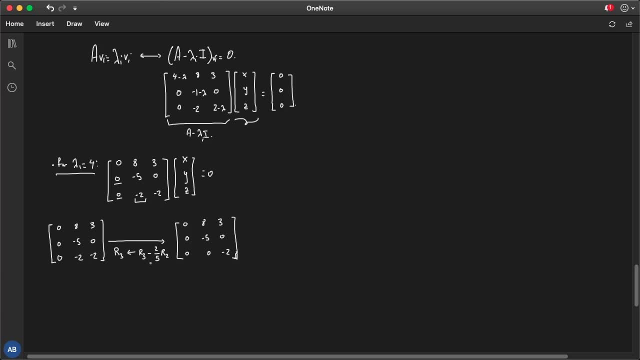 That is, any row operation done on the matrix will give us the same solution. So we're still solving for the same system written differently, And the most efficient way to solve it is by back substitution. So what you get from this system is that starting. 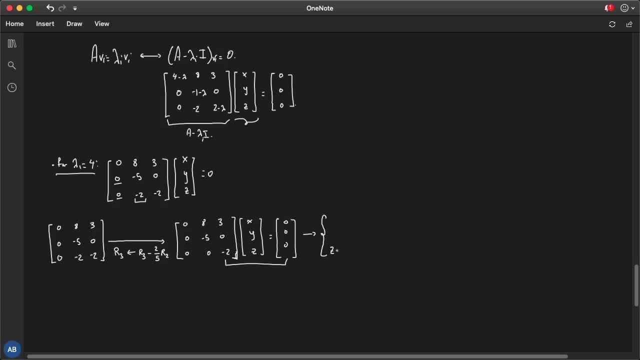 from the last equation we get that z is zero. Also, this equation gives us that y is zero, Whereas the first system gives us that x is free to move in R. okay, So any value of x would do. We're going to pick x to be one. 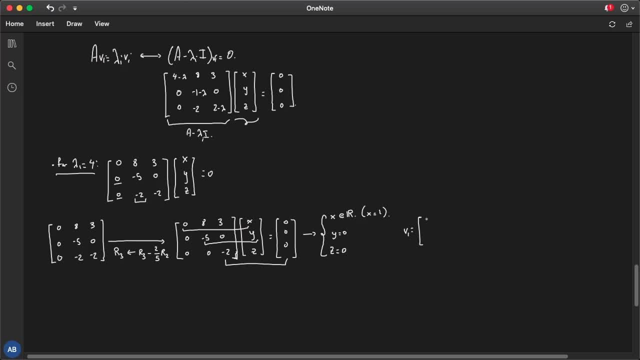 and hence the eigenvector is one, zero, zero, right. So this eigenvector corresponds to the eigenvalue, and we're going to do the same thing for lambda one equal to four. Now, the same thing here, for we're going to do the same thing. 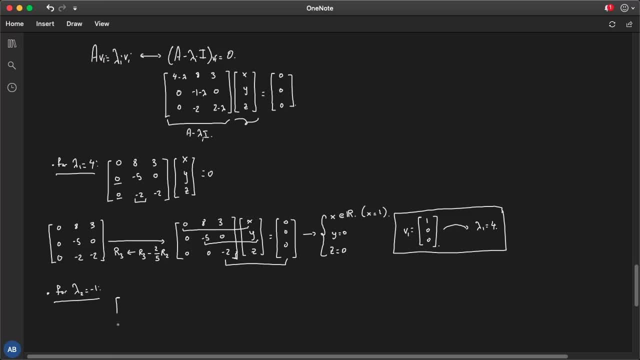 for lambda two, that is minus one. What we get is the following system: So instead of lambda, we plug in minus one over in the A minus lambda I matrix, We get five, eight, three all zeros and zero minus two. 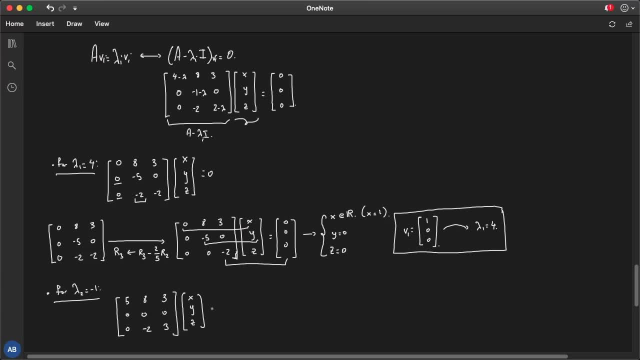 and three. Multiply it with x, y, z to get all zeros. So this system is very easy. This system is easily solved. The second equation doesn't give us anything. The last equation gives us that y should be three over two z. 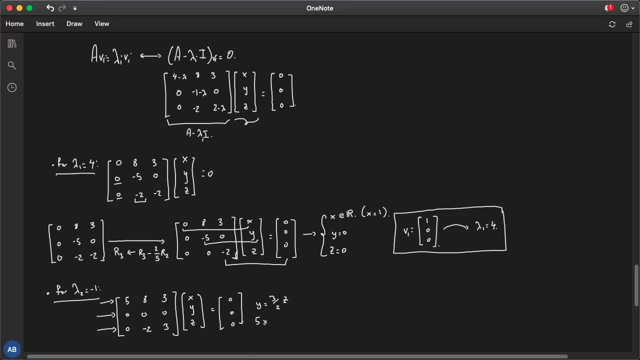 And the first equation gives us that five x plus eight y plus three z is zero. right, Placing equation one and equation two, we get that five x is minus 15 z, That z is zero, That x is minus three z right. 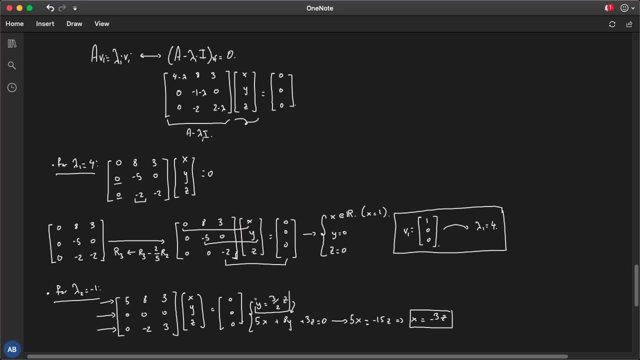 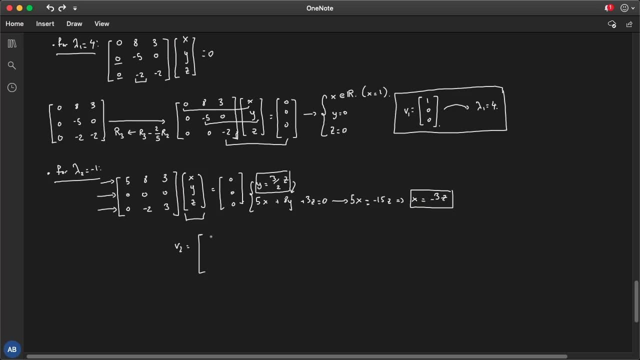 So this is x in terms of z and this is y in terms of z. So the eigenvector that we're looking for is actually of the form x, so parametrized in terms of z. So x is minus three z. 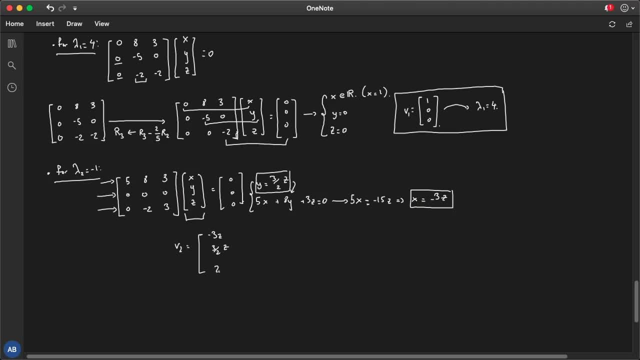 Y is three over two, z and z is z right. So for z equal to one, we get minus three, three over two and one. So this is one possible eigenvector corresponding to lambda. two is minus one. okay. 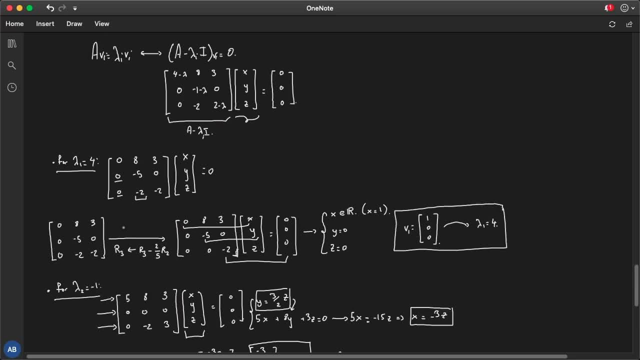 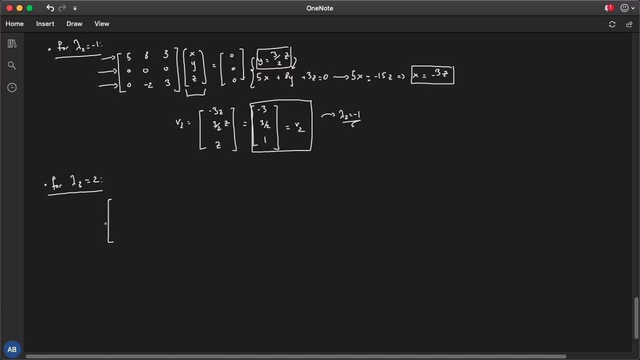 Now for the last eigenvalue, that is lambda. three equal two. we replace this value in a minus lambda i to get two, a three. zero minus three zero and zero minus two zero. The way you can solve is whatever way really. 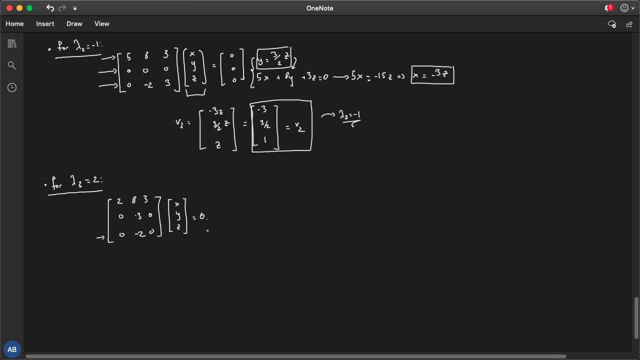 So this equation gives us that y is zero and this equation gives us the same thing. So you get that y is zero, Plugging it in the first equation, that is two x plus eight y plus three z. So this guy goes out. 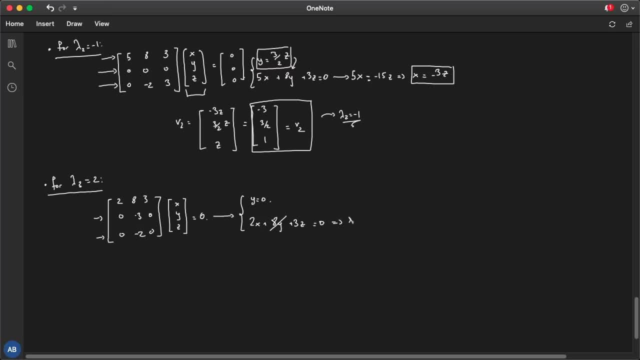 This is zero. You get that x is minus three over two z. okay, And y is zero. So the eigenvector, right, The eigenvector we're looking for, v three is actually of the form minus three over two z. 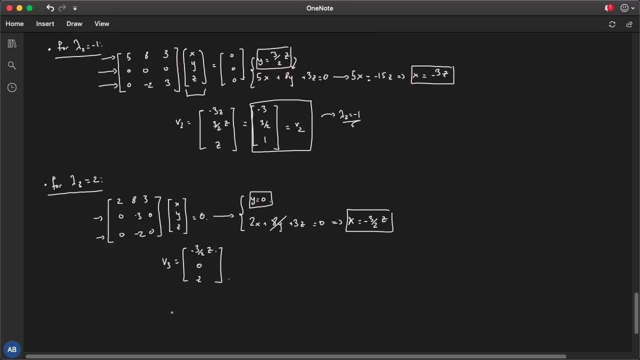 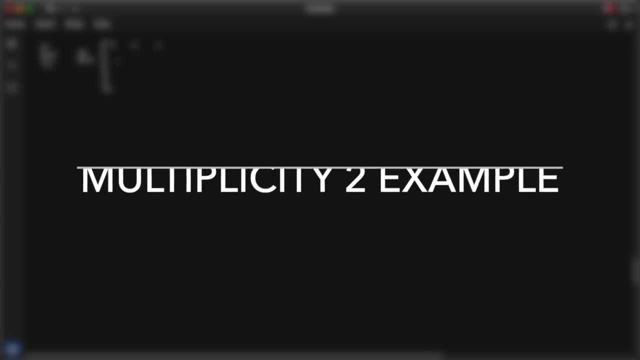 y is zero and z is z. For z equal to one, we get a possible eigenvector that is associated to lambda. two is equal to two. One last example is on the matrix A, that is the all ones matrix, So one everywhere. 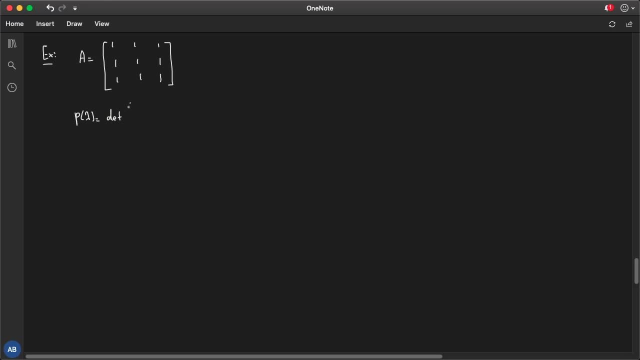 Writing down the characteristic equation that is the determinant of A minus lambda i, which you can write down as lambda square into lambda minus three. That means that lambda equals zero is of multiplicity two and lambda equal three. Well, in this case, 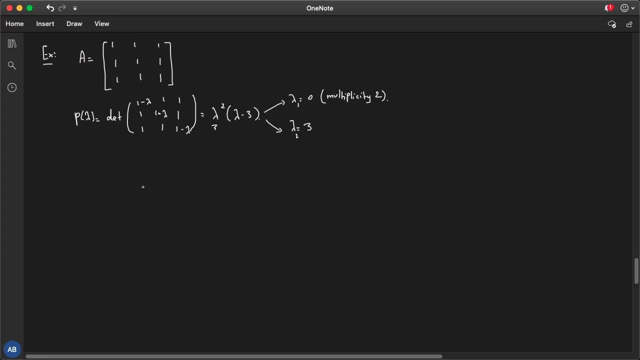 if we want to find the eigenvector corresponding to lambda equals zero, what do we get? So for lambda equals zero, we get that A minus lambda i is of the form one, one, one, one, one one, All ones. 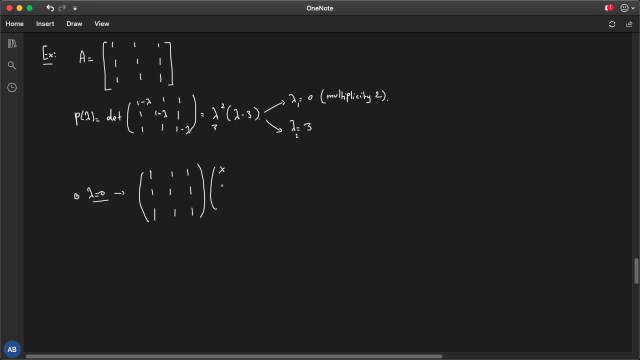 so a, in other words, multiplied by v, this guy is v is all zeros. so using gaussian elimination we can do some row operations to get the following matrix: which means that x is minus y minus z from the first equation, and that's it. that's all the equations. you get the second and third equations.